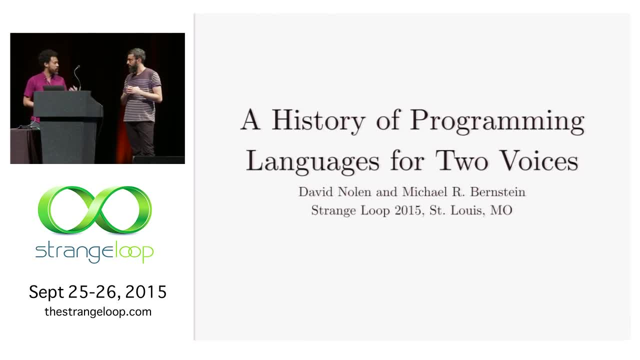 to present this talk. It's something that we kind of got together. We both have a very deep love of programming languages, But we're also really we're musicians, but we're also sort of music connoisseurs, so to speak. So we thought it would be cool to do basically. 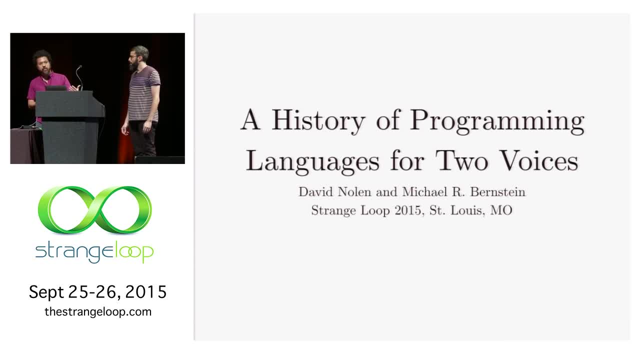 it's kind of like a mixtape about sort of the chronology of programming languages, along with interesting things that were happening in music around the same time, And kind of like a mixtape. we're kind of juxtaposing things. It might not even be clear exactly. 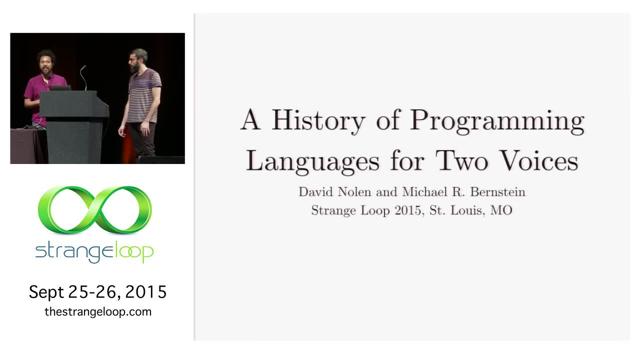 how these things are related, But hopefully it's going to be interesting, It'll create maybe interesting ideas and it'll be a lot of fun. So a little bit about myself before we get started. My name is David Nolan. I am the lead developer of ClosureScript. 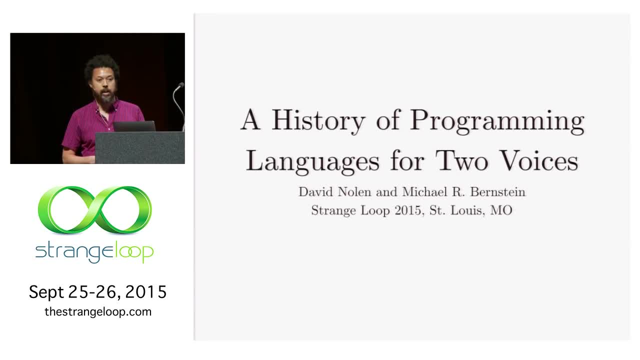 I also work. I'm a software engineer at Cognitech. I work on Datomic, which is a mutable relational database. Hi, I'm Mike Bernstein. I'm an amateur computer scientist and record collector. I work for a company called Code Climate That's based in New York City. It's a hosted static analysis. 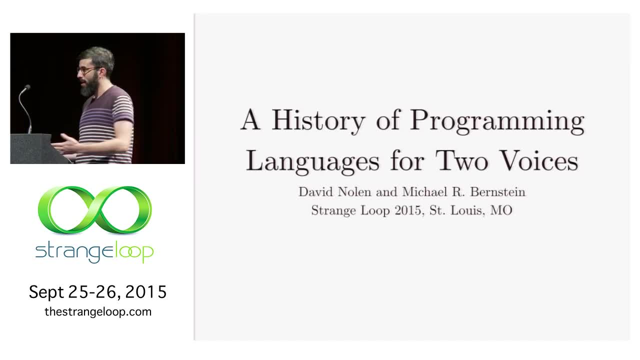 platform And we should get started. Like David said, New York One thing is, talk is not, isn't comprehensive. So, in the same way that you probably wouldn't yell at your high school boyfriend for making you a mixtape that didn't have every single- 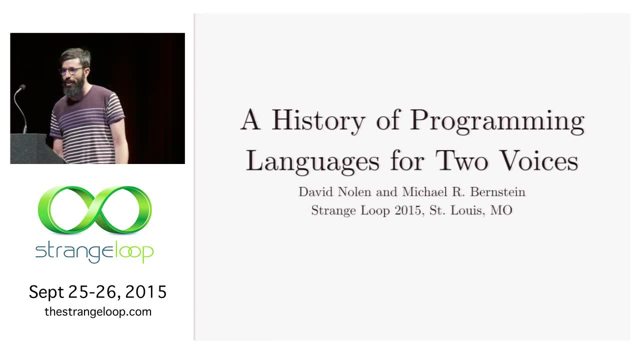 song on every single album on it. don't expect more than what you see up here. We're really excited to present to you today and a little bit like two seconds of off script. I just wanted to take an opportunity to really thank Alex Miller for putting this conference together, and all the organizers, and particularly 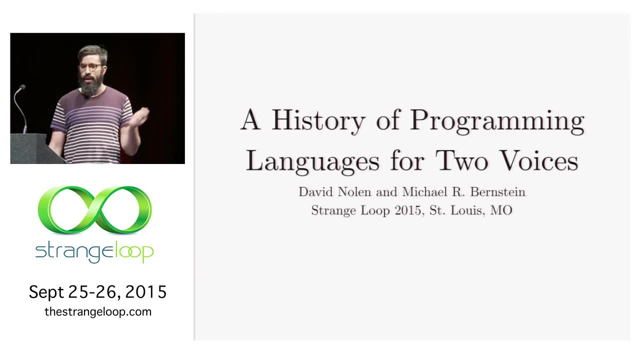 for inviting Alex Miller. Excellent Thanks, Mike. We hope to see you soon, Thanks, Bye. Thanks, Dave. last night's closing keynote to speak. The issues that were addressed in that talk are extremely personal and important to David and I. 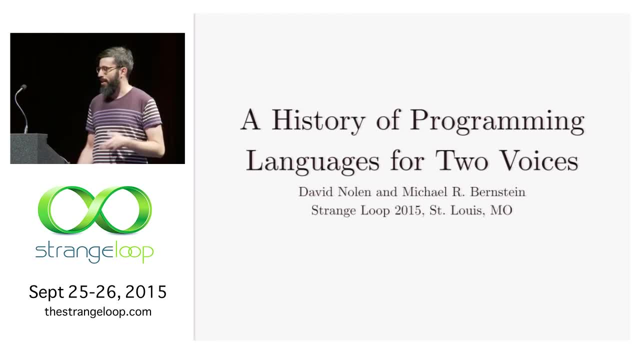 and we were saying before yesterday that this is our favorite conference and having something like that here really nailed that home. So on to the talk. The talk is: thanks, yeah, So we've divided the talk into a few different sections. 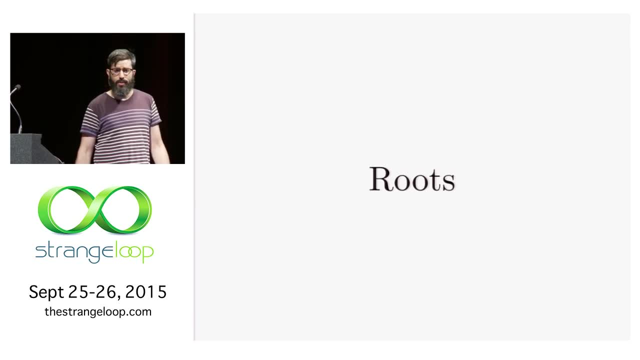 You know, the history of music is much longer than the history of programming languages, and so, since this is our idiosyncratic mixtape, we decided to start in a section that we call the roots, and the roots of computer science. 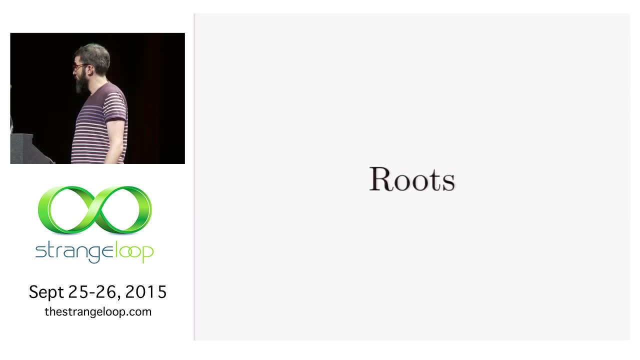 that we decided to start with were in around the mid-1930s or so, and this is where we're going to begin our journey and David's gonna start us off. So part of the reason why we were starting sort of in the 1930s is that I mean. 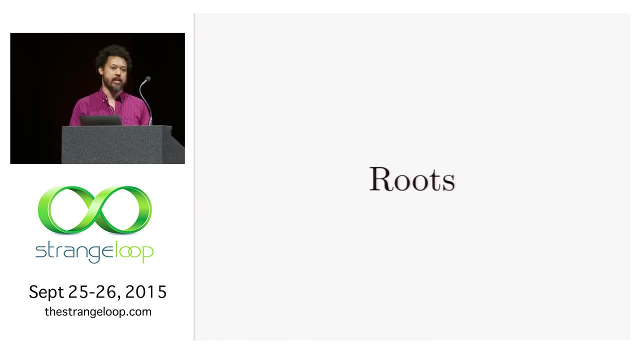 if you really look at a history of computing. I mean, there's so much history around mathematics and logic, but it really wasn't until the 20th century when people started coming up with computable theory, when the fact that computers could even be constructed. 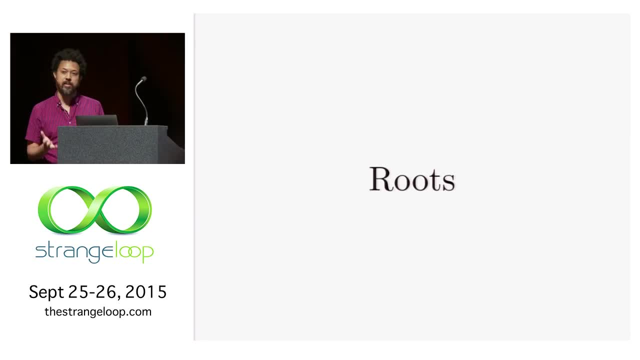 and that software was actually gonna happen. that computing really took off. It's very much a 20th century phenomenon- computers- But in a similar way, something happened to music around the same time, and this was the ability to record music onto some physical thing. 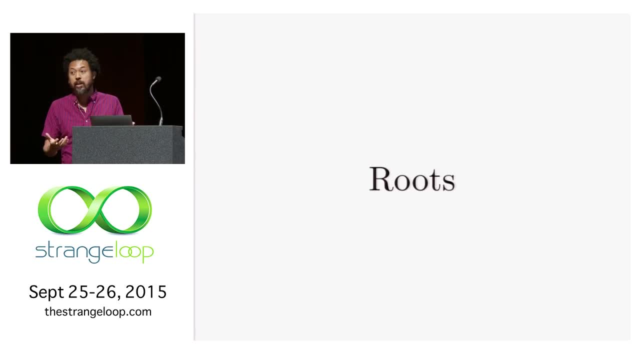 and distribute that music Prior to the 20th century. you really couldn't, you know, experience music without either being able to perform it yourself or being in the presence of a performer, and I think it's easy to see that music. 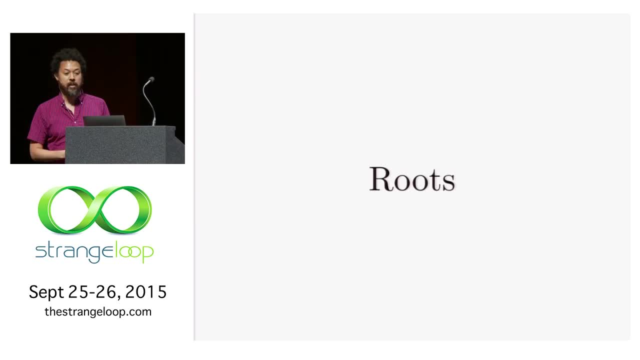 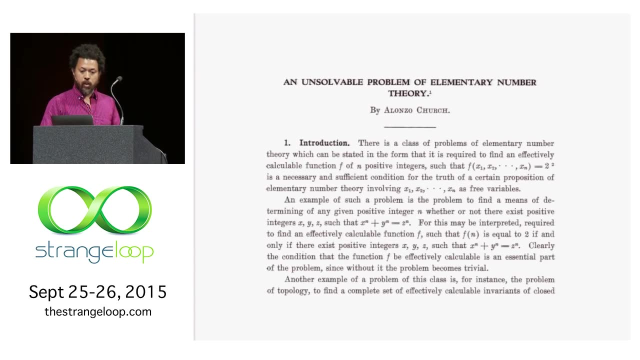 I mean, music has always been an extremely important part of human life. but you've seen it explode in a way that I don't think anybody could have predicted, thanks to recorded music. So you know, for the computer science stuff I mean, you could pick a lot of places to start. 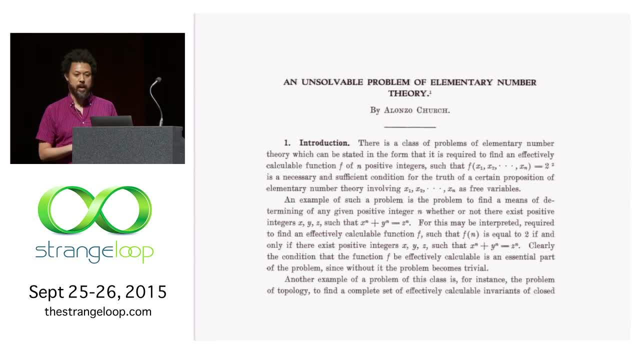 but we're both fans of functional programming and this is such a huge paper. This is where Alonzo Church was sort of thinking about computability and he sort of, on the side, invents this thing called the Lambda Calculus. And you know that will trigger a massive, you know, development in theory. 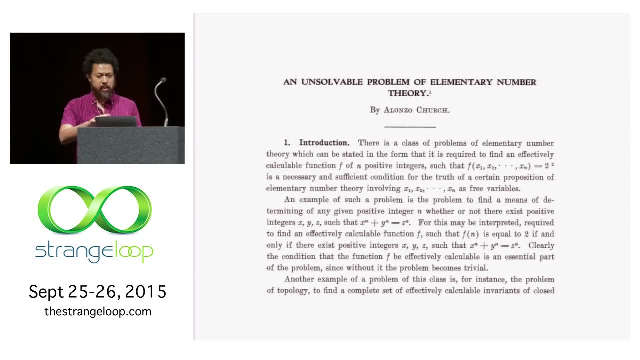 But as well as something that people couldn't have imagined. you know, almost 30 years after this, somebody would create a programming language which would use the Lambda Calculus as its foundation. So you know, this is the beginning of a very big bang. 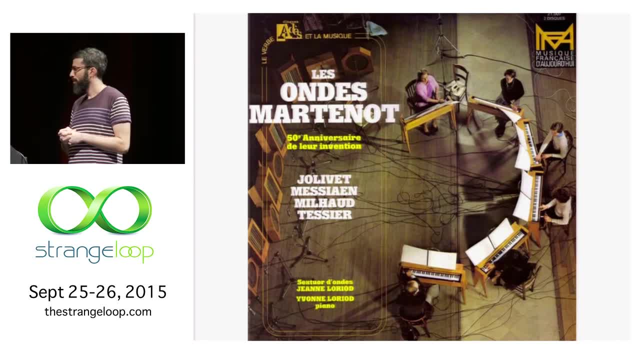 We like to say the Lambda Calculus. You may have heard of it, So we picked this record. It's a really cool record. This is a collection of pieces by 20th century composers. Quite a few interesting people on this one. 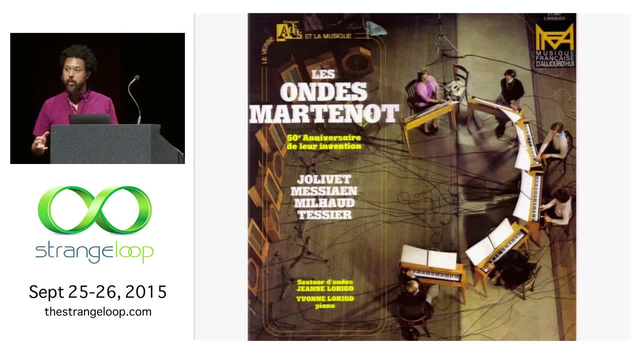 The one we're going to play for you is Olivier Messiaen. He was a serial composer but he really loved birdsong And he wrote pieces specifically for this new type of instrument And it was kind of like a theremin, but it had. 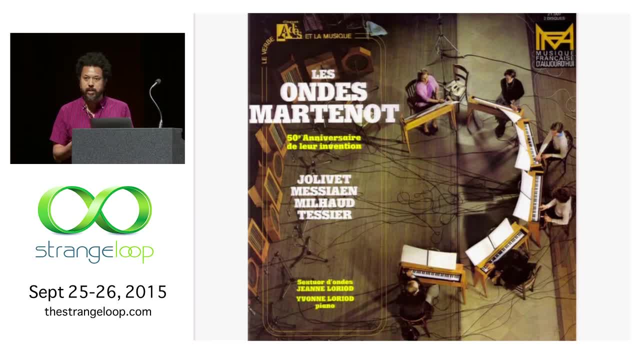 keys And it had a very- to me, a very- 20th century sound. It's electronic, It's something that people really hadn't heard before. We're going to play you a short clip of this. So the reason why we chose that, as David said, is that that doesn't sound like music. 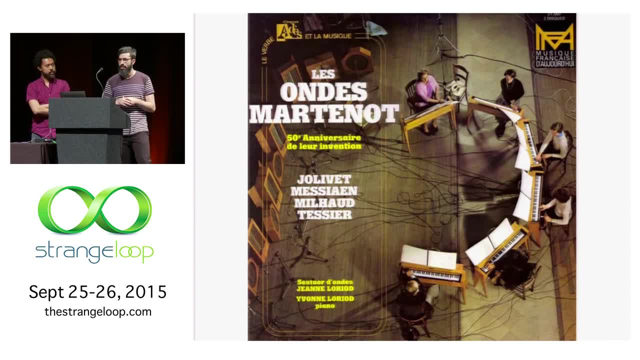 that would have been composed in the early 19th or in the early 20th century, to me anyway. So having an individual that composes music start to look for other media through which to express their sound was a really profound and interesting thing to us. 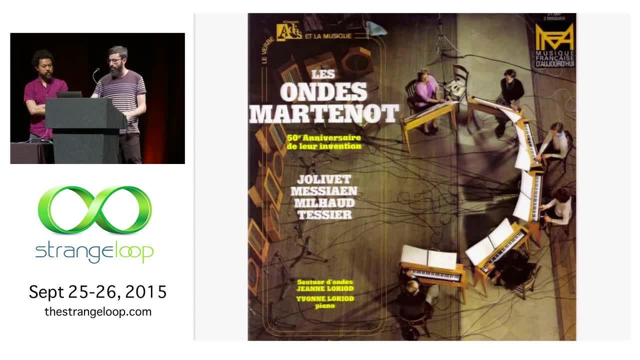 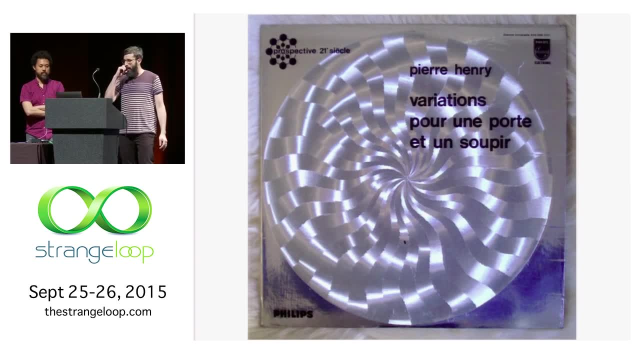 And there are echoes in what David said about programming languages in this music. And we're going to play one more piece from the same record. This is a piece from the same record. This is a piece from the same time period, roughly. This is music by Pierre Henry that he composed with his mentor, Pierre Schaeffer, in France. 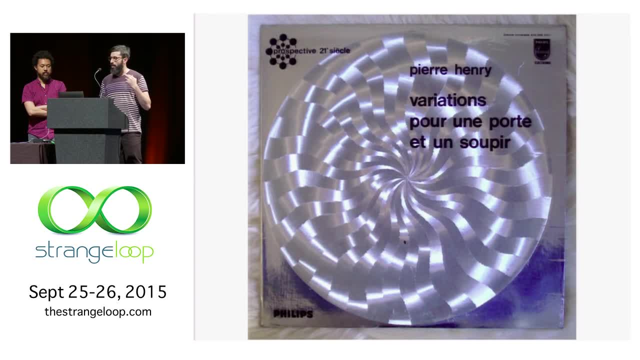 And they invented a genre of ostensibly contemporary classical music called Musique Concrete. So they take this idea of using pure electronic media to express music even further by removing all instrumentation from music and composing only with tape. So most people conceive of the idea of sampling as being: you know a late, you know early. 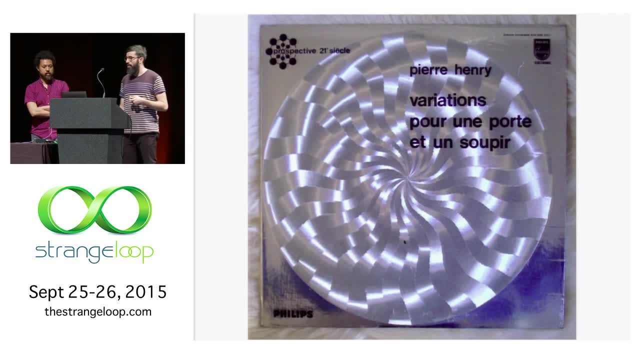 music. It's not a 1920th century phenomenon, but in fact these gentlemen in suits and very serious faces in the 1930s and 1940s were making music that a lot of people might take issue with calling it music. 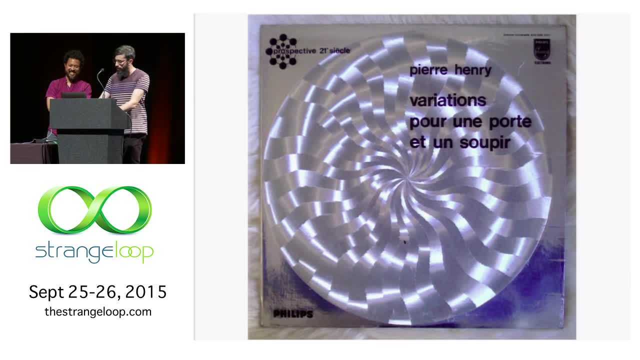 So let's hear Variations on a Door and a Sigh, And the reason why it has that title will be very clear: It's OK to laugh. It's OK to laugh, Hmm-mm-mm, OK, Mm-hmm, Yeah. 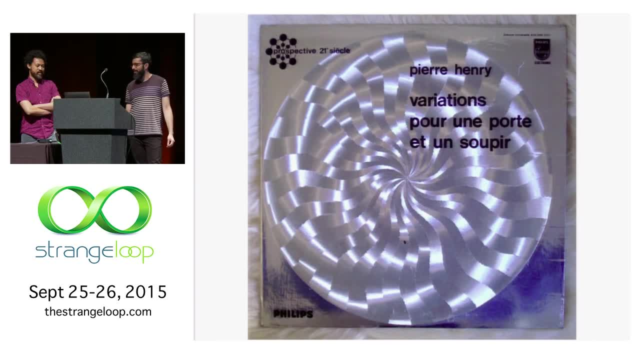 Mm-hmm, Yeah, Mm-hmm, Comedic timing. So that is a piece of music composed of the sound of a door kind of creaking and a person sighing, And they took these samples on magnetic tape and manipulated them in all these different 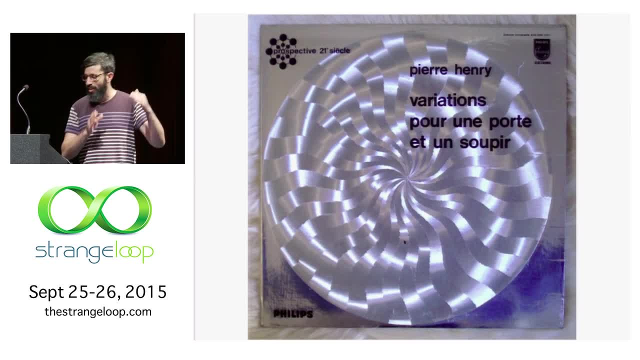 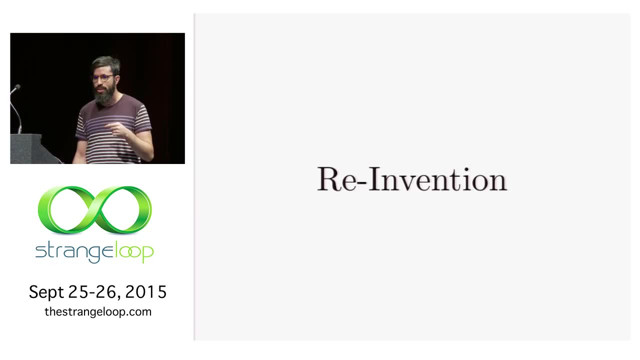 ways and from that they made their composition. And this leads us right into the next section that we call reinvention. And the idea for this section in reinvention came from that, you know from the between the early 1940s and the mid 1950s, you know, actual computers were invented right. 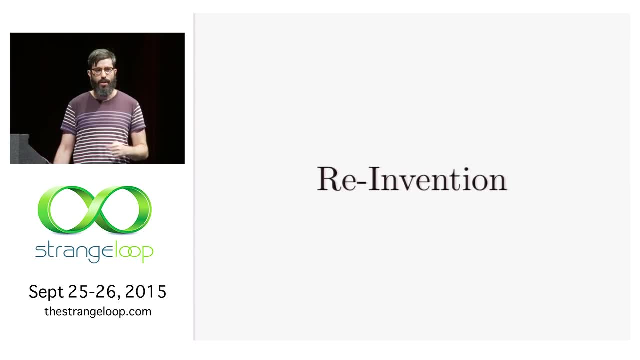 So you had like actual machines that people could program things on. It wasn't a very pleasant experience to program them, But by the time we get to this period we see people taking the actual material of computation and thinking: hmm, I wonder if there's a different way that we can do that. 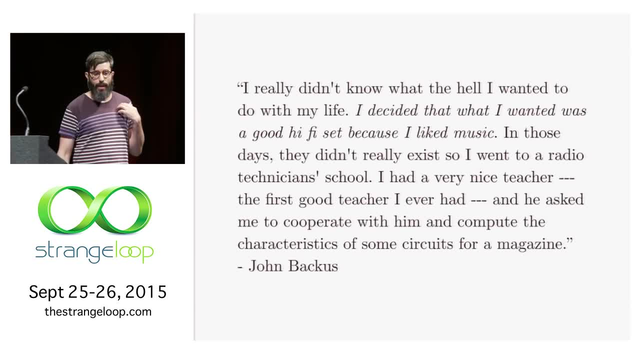 And we're going to start this section off with a quote from an interview with John Bacchus, one of the inventors of the Fortran programming language, excuse me. and he said: I really didn't know what the hell I wanted to do with my life. 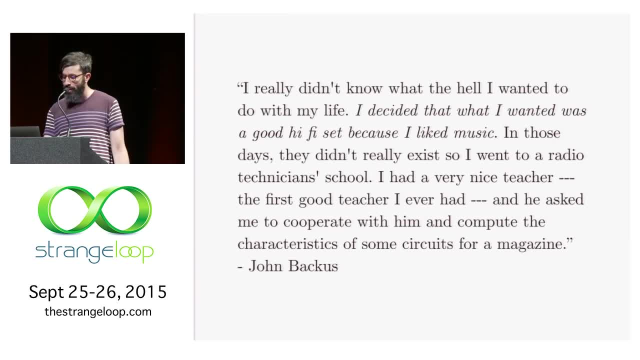 I decided that what I wanted was a good hi-fi set because I liked music In those days. they didn't really exist. It's interesting that he wanted one if they didn't really exist. So I went to a radio technician school. I had a very nice teacher- the first good teacher I ever had- and he asked me to cooperate. 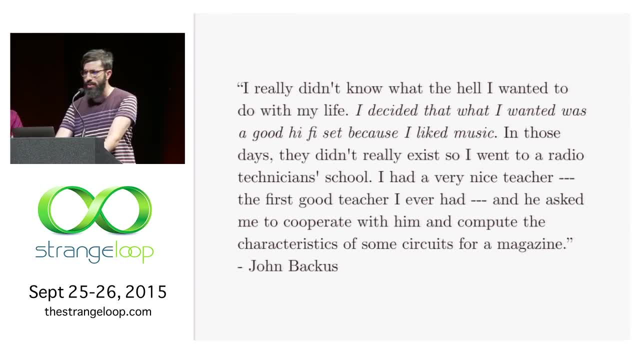 with him and compute the characteristics of sound. He said: do you know how to do it? And I said I don't know. And he said: well, I'll teach you how to do it. And he said: well, it sounds really cool. 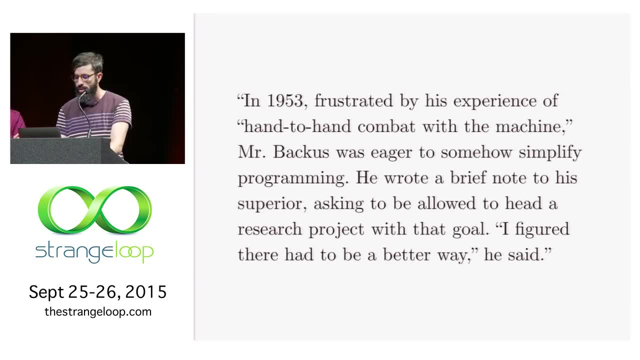 It's a good idea. I said OK. So I wrote a book about sound. It was a pretty interesting book, But there was some circuits for a magazine. So he kind of fell backwards into computing And, as you'll see, he didn't find it to be a particularly pleasant experience, as you. 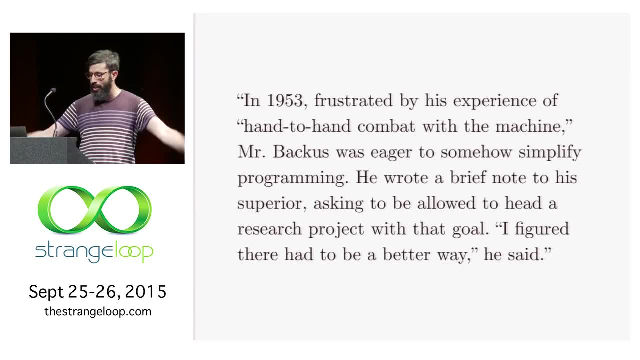 see in this quote from the same interview. In 1953, frustrated by his experience of hand to hand combat with the machine, Bacchus was eager to somehow simplify programming. He wrote a brief note to his superior asking to be allowed to head a research project with 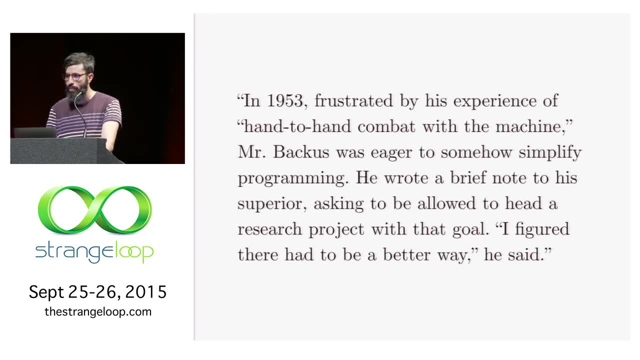 that goal. I figured there had to be a better way. he said- And we think this is still true- right, And this is one of the themes of this talk- There's always, we think, going to be a better way. 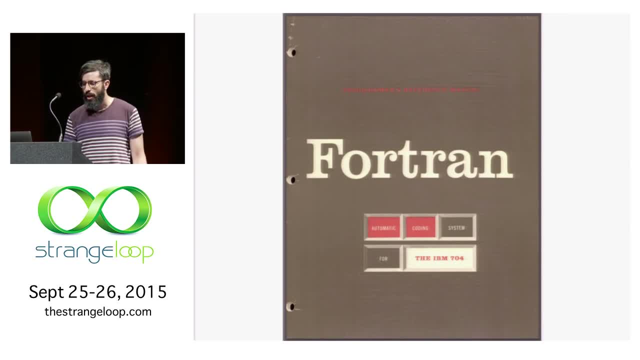 And so he made a better way. It was called Fortran, And this is the front page of the Fortran manual, designed to run on the IBM 704 in 58,, 59, or something like that, And here you have a high-level programming language. 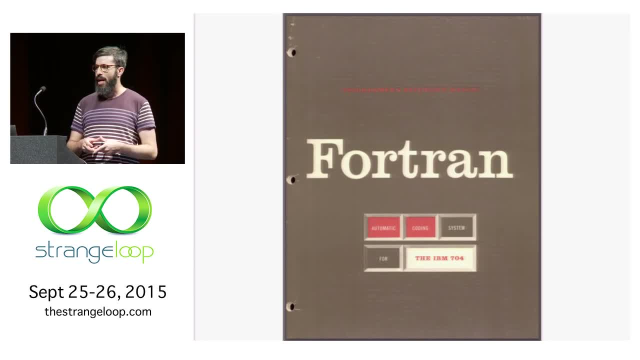 designed for scientific computation that allowed people to actually use things like abstraction in order to express algorithms and programs. So this is that reinvention that we're talking about, And we're going to hear about two more languages that were created around the same time that similarly harnessed this desire to program computers. 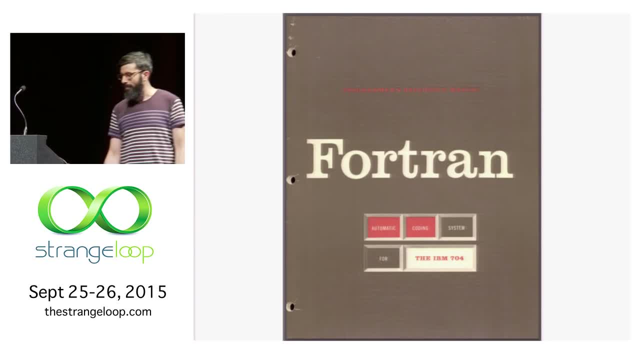 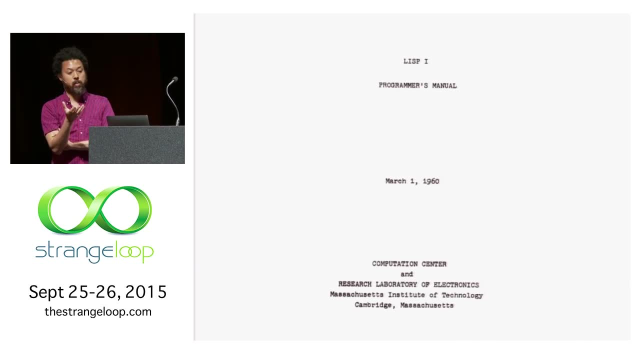 and not necessarily fistfight with them. So shortly after Fortran appeared, John McCarthy invented Lisp. That was in 57.. This is a page from the Lisp 1 programmer's manual. It's dated March 1, 1960.. And this is actually a manual that talks about Lisp 1. 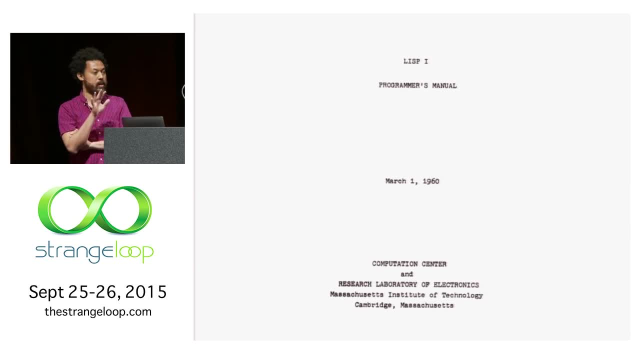 to run on the IBM 704.. So this was the promise of compilers generating the assembly code for a particular hardware was actually happening. People could program in higher-level languages at a higher level of abstraction and get something done. What's fascinating about this is that two compilers 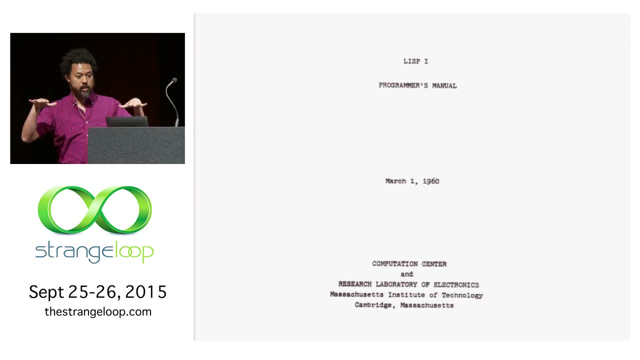 or, in this case, an interpreter with some sort of runtime. still, the idea was a common desire, a high-level program, but so different in their manifestation. Fortran was about technical computing like calculation, And Lisp was created by a sort of a mathematician, a logician. 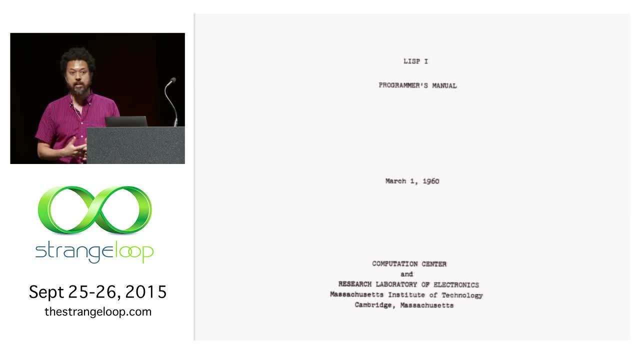 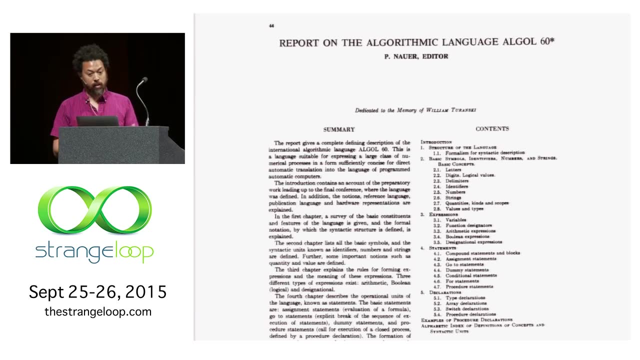 And he wanted to do something very different, which was symbolic mathematics, specifically to pursue this thing that he was calling artificial intelligence. Shortly thereafter, in a couple more years, a bunch of smart people got together and they created Algol 60. And the shadow of Algol 60 is vast. 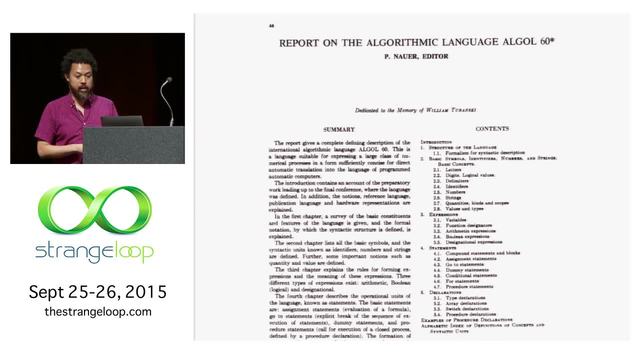 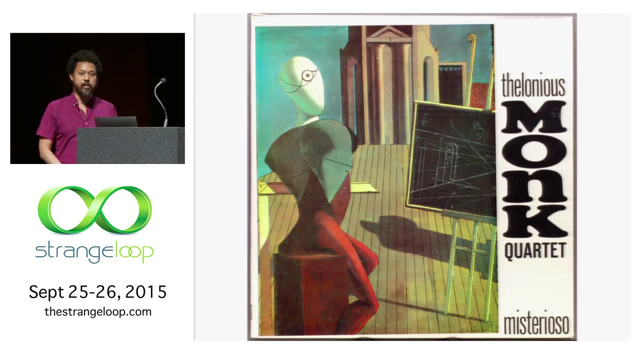 Almost everyone, almost all of the programs in some dialect of Algol 60. It's the most popular sort of dialect that exists today. So when we were sitting around talking about what music should we pick that makes sense or has some sort of relationship to this period of time? 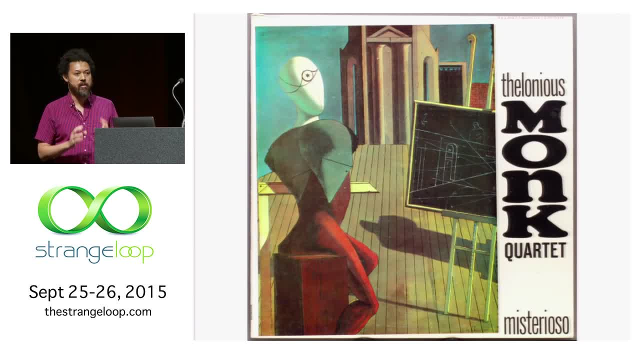 and we sort of settled on the jazz movement in the 50s. And the reason we did this was because, in the same way that computing had already existed for a good 30 years, right the idea of computing, the theory of computing, 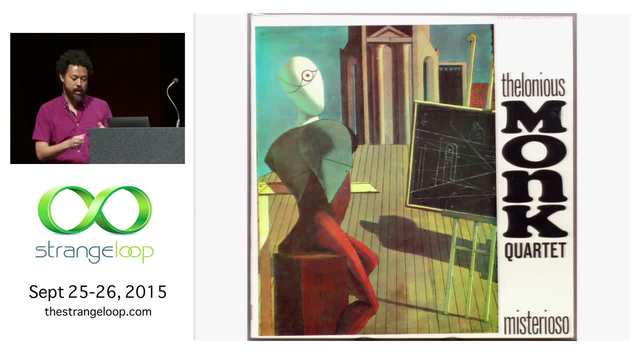 actual computers and programming languages. This was happening And the compiler thing and the interpreter thing really sort of you know, allowed computing to become sort of kind of free Jazz had been around for 40, 30 years already, But in this period a bunch of talented individuals decided. 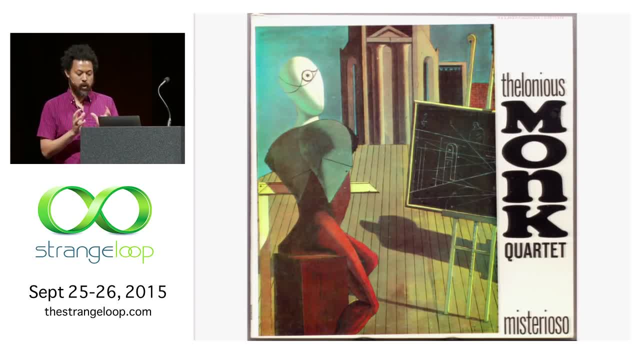 to distill jazz into a very, you know, pure essence, And I think Mike has some more things to say about that. Mike Stebbins- Yeah, so we're going to play you a sample from a pianist named Thelonious Monk, who's often considered one. 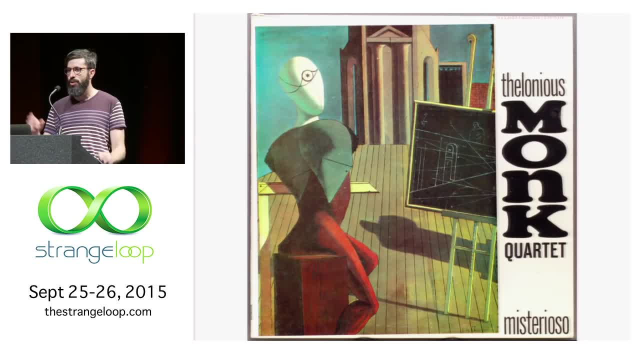 of the greatest jazz pianists and composers of all time And in fact, was one of the progenitors of this new style of jazz called bebop, and then hard bop and post bop and all of those kinds of things. So this is what we want you to listen to in this music. 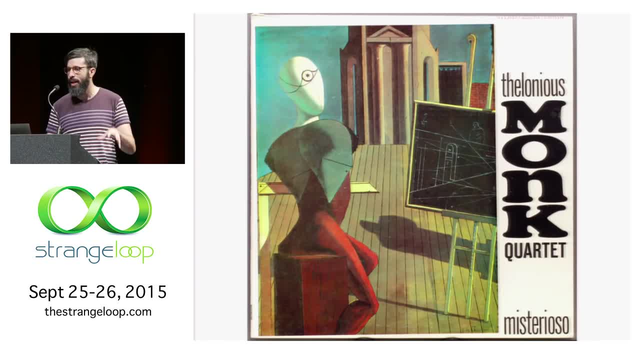 if you don't know jazz and you've never heard it before, is just listen to the piano. listen to the rhythm of the piano and the way that the piano is interacting with the music. This is a live recording from the Five Spot in New York City. 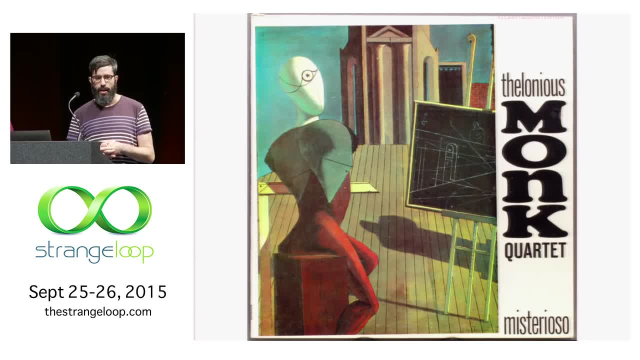 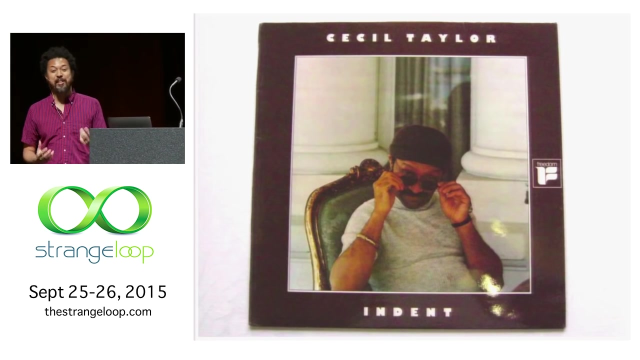 And it's a tune called In Walked Bud that Thelonious Monk wrote and dedicated to his music, His pal Bud Powell. It's one of my favorite pieces of music. It's a really nice piece. Yet another pianist, but very, very different, is Cecil Taylor. 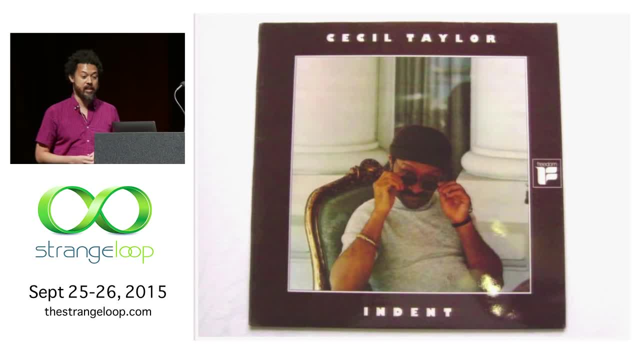 So Mike and I are both lucky enough to have actually seen Cecil Taylor perform in New York. Cecil Taylor was really somebody of the 60s and 70s, but he started in the sort of bebop scene in New York City. What's interesting about the way that he plays is that it's very percussive. 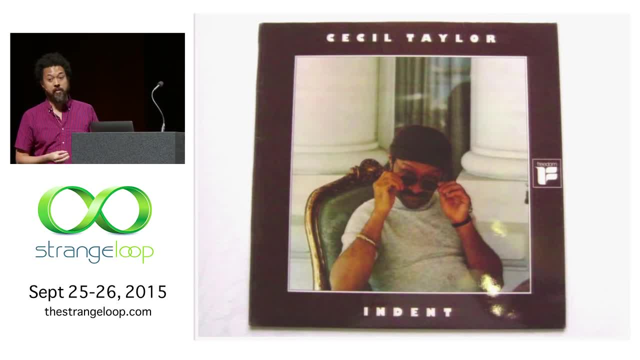 He was really a big figure in what's called the Free Jazz Movement, which was a distinctly African-American intellectual sort of event. that happened, which is fantastic. Most people know Ornette Coleman. Not as many people know Cecil Taylor. What's really cool about his music? it's so much distinctly his own thing. 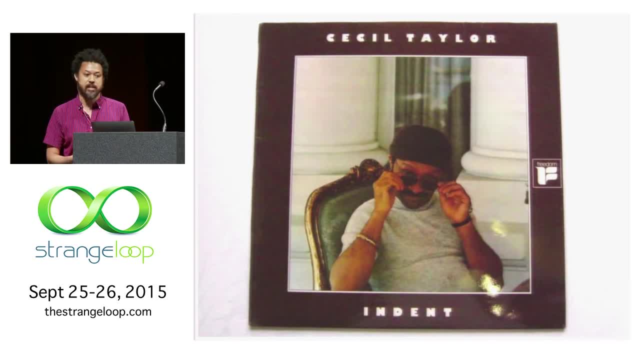 yet it's still jazz. Again, you'll hear that it's very dissonant, very rhythmic, very percussive. It's almost like he's drumming the pianos ¦ ¦, ¦, ¦, ¦, ¦. 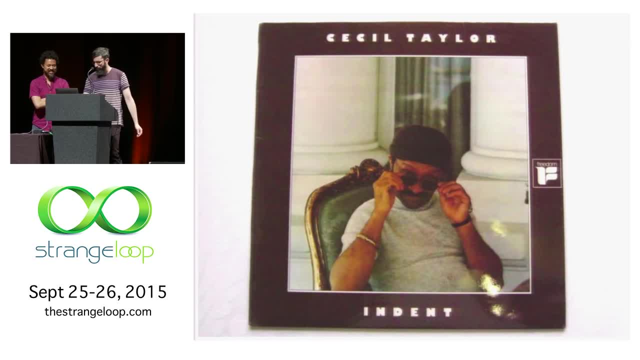 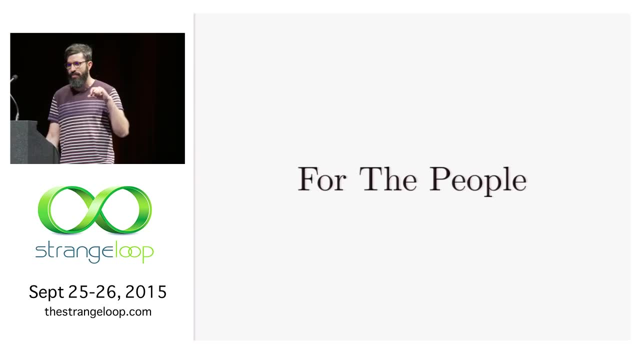 ¦, ¦, ¦, ¦, ¦, ¦, ¦, ¦, ¦, ¦, ¦, ¦, ¦, ¦, ¦, ¦, ¦ ¦ 70s. So in the mid-1960s you see a movement where populism and popular culture really 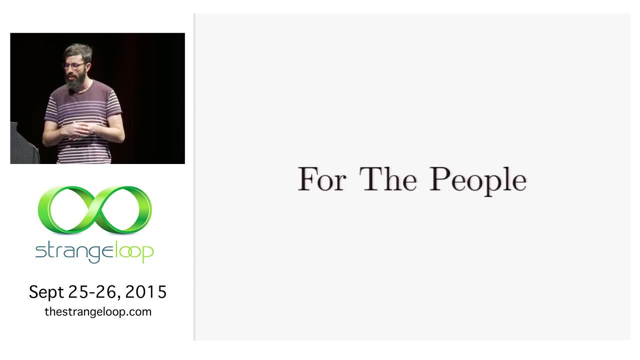 starts to take hold in a really interesting way, especially in the United States. So we're going to see an example of one programming language that we feel fits this bill, and then a piece of music as well, And David's going to talk about BASIC. 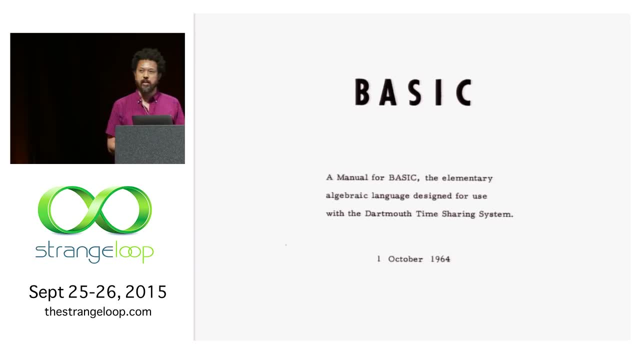 So a lot of things happened in the 60s. We're only going to focus on this one, because I think it drives a really just important point home, which was an attempt to expand the number of people that could get access to the power of computing. We found this: This is a BASIC. 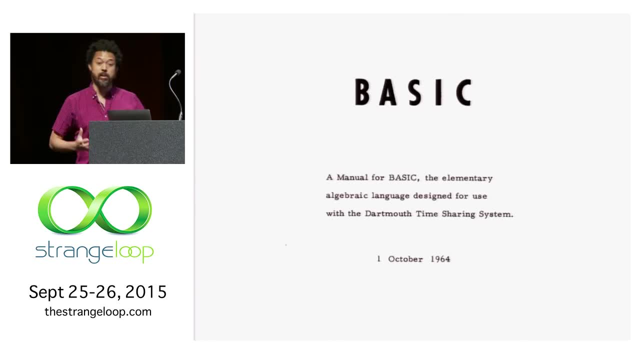 user manual from October 1964.. And the introductory paragraphs in this is really incredible. While Fortran might be great if you're a scientist and LIS might be great if you're a logician, there are lots of tasks that computers can help humans accomplish that don't require 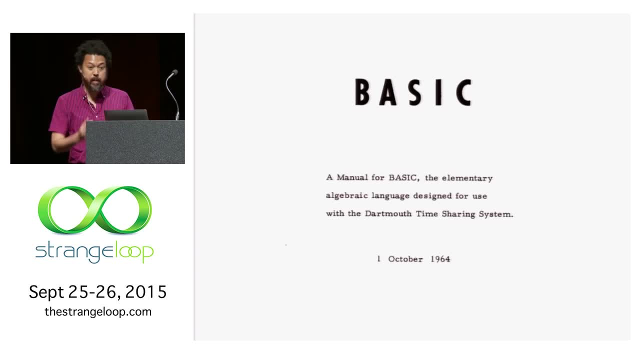 that level of sophistication. And the beginning of this manual basically says: almost anybody can pick this up. You know, you can look at this manual. you know, spend about a week and you'll really be able to get it. And the truth is, I know there's probably a lot. 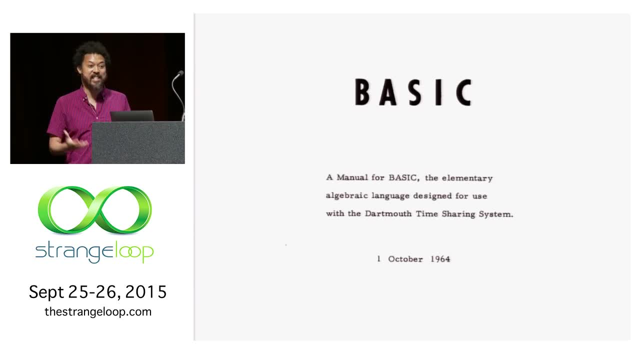 of you in the audience that probably learned BASIC when you were children. right, BASIC is simple enough for a child to pick up And I think to this day, people are constantly looking at ways to widen the scope of people who have access to the power of computation. 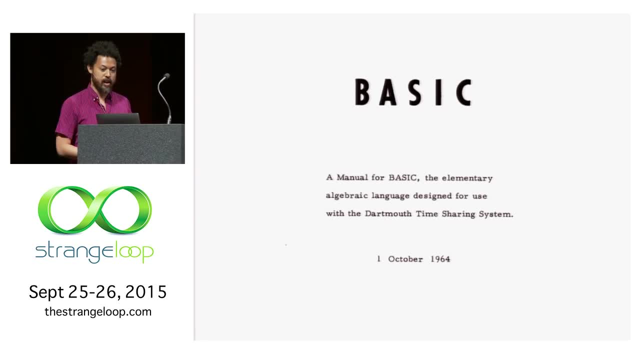 So this is why I sort of thought: BASIC is the language of the people And Mike's going to talk about the music selection. MIKE HOLLANDERMANN, Yeah, so there's a lot of amazing music from this period of time, But 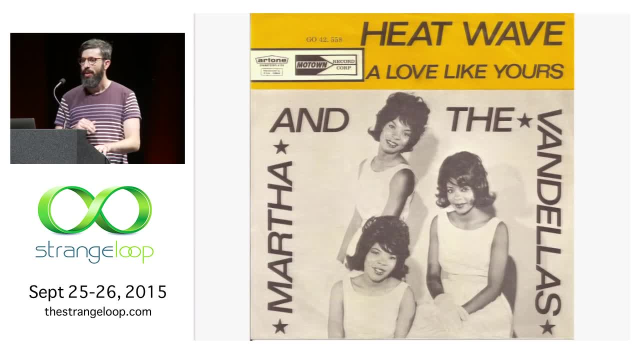 one thing that I think is really important is that we're going to be able to pick up a lot of music from this period of time, But one thing that we couldn't ignore was Motown. So in the mid-1960s, you have a movement that starts in Detroit based around a record. 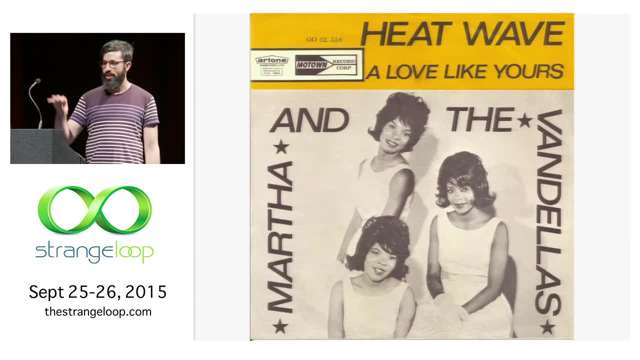 label, And this is one of those record labels that has a sound right. These producers and musicians and songwriters collaborated to make something new right To make a from-the-ground-up new sound that ended up being one of the most important and enduring popular music movements. 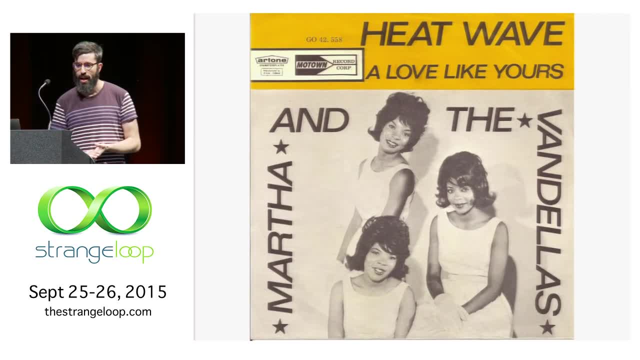 ever, right, MIKE HOLLANDERMANN, Right, MIKE HOLLANDERMANN. I think everyone loves Motown music And one of my favorite Motown tracks is Martha and the Vandellas Heat Wave, And it's OK to Dance to this song if you. 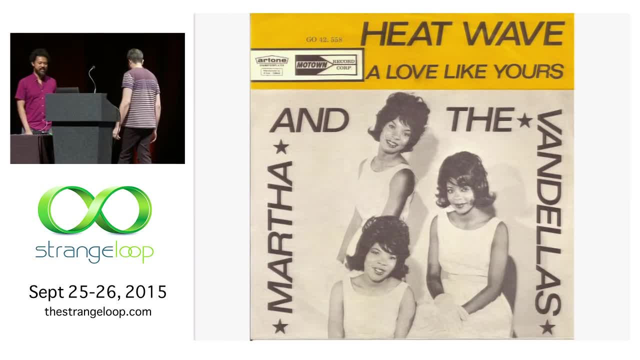 have to MARTHA AND THE VANDELLA. Whenever I'm with him, something inside starts to burn me and I'm filled with desire. Could it be a devil in me, or is this the way it's supposed to be? It's just the way it's supposed to be. 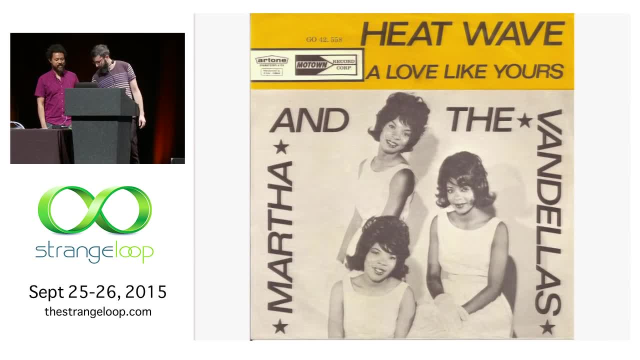 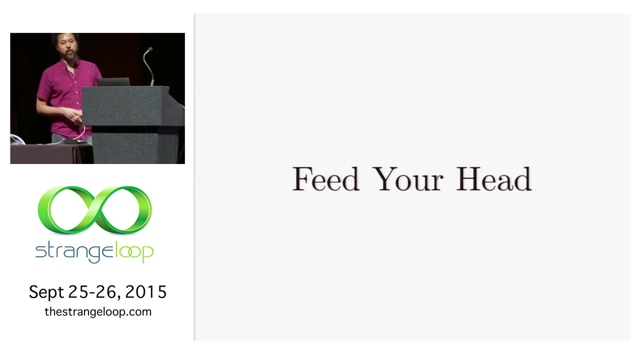 So the next section is called Feed Your Head. We're moving into, you know, the psychedelic 60s. There was a lot of civil unrest all around the world. People were questioning you know the way that society was organized, Really sort of shaking things up. 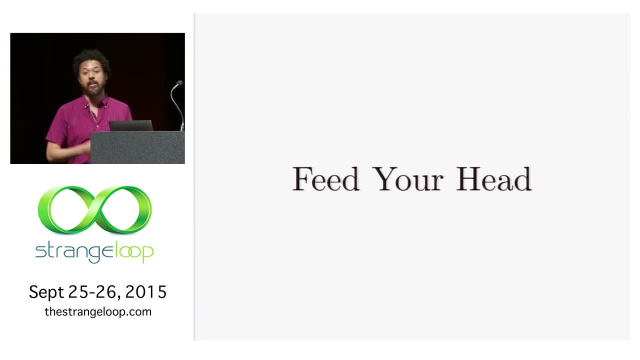 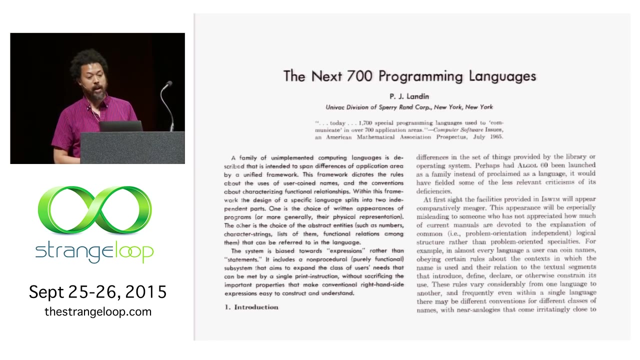 You see a similar thing happening in computer science. People had lived now with programming languages for quite a bit of time And people were starting to really go back and revisit some of these assumptions and early designs. There's a very famous paper by Landon called The Next 700 Programming Languages. 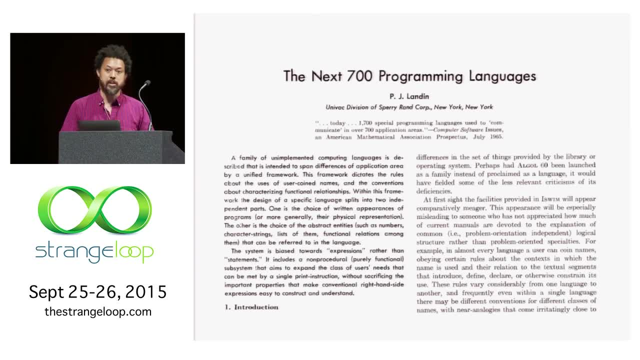 And it's really sort of looking at. you know, while we understand that high-level programming is very effective, it became clear that even when you have a high-level programming language, there can be flaws in the design, there can be problems with the semantics. 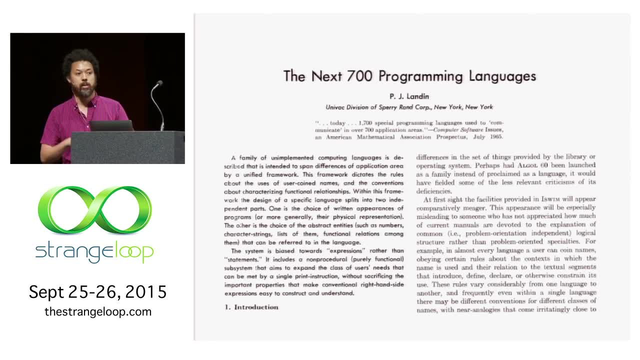 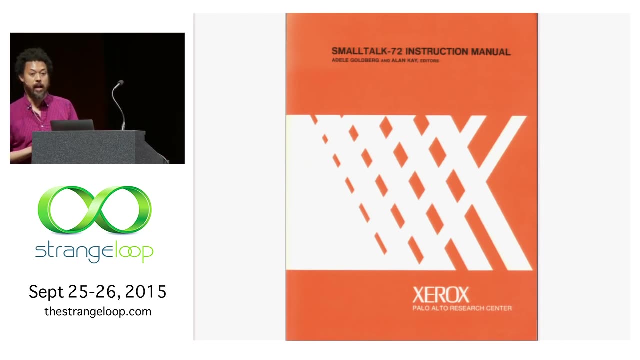 He refers to something in this paper called iSwim, which will in many ways, be the spiritual predecessor to things like Miranda and Haskell. So you get a sense that people are looking for something new. A lot of people started working on doing new things. 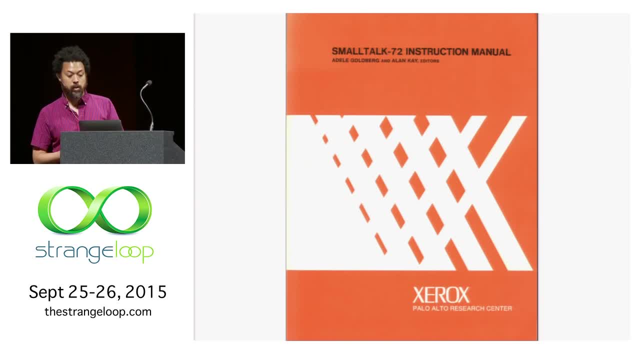 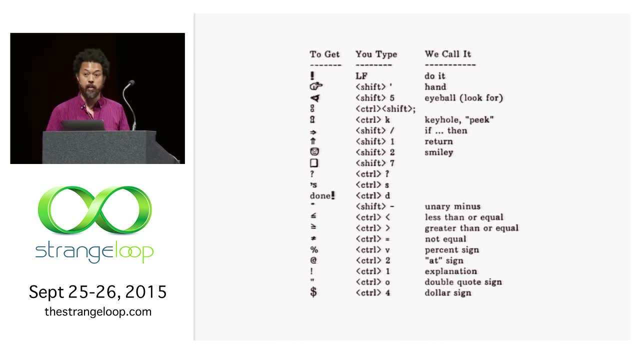 Alan Kay at Xerox PARC invented this language called Smalltalk, which also ended up having a very long shadow. Its early incarnation, though, was far more radical than how Smalltalk 80 ended up. Smalltalk was a language that was designed to be oriented around many things that people 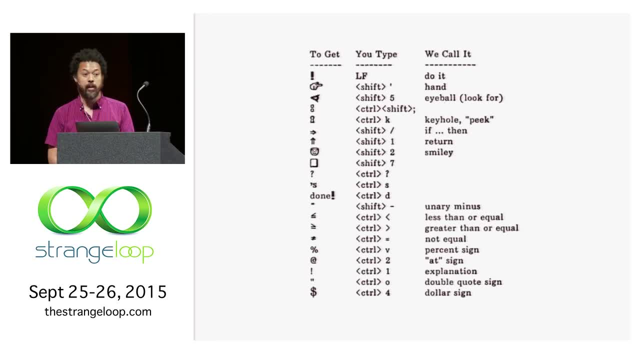 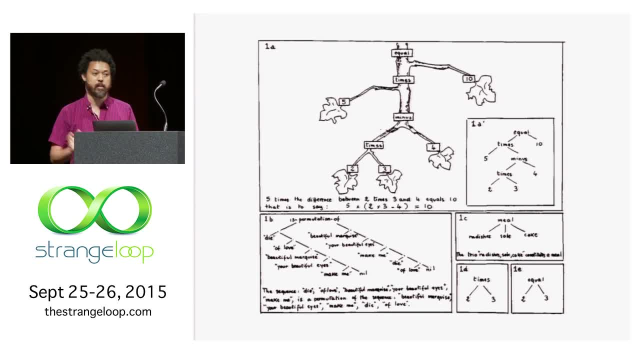 And then you also had things like Alain Comeran and his group. they created something called Prolog. Right Up to this time, people were writing imperative algorithms and really sort of instructing the computer, step by step, what needed to be done. 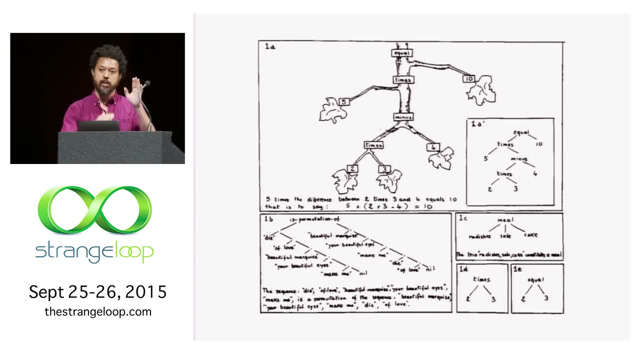 But Prolog had this totally radical idea: whereas you make a series of declarative statements and then a search algorithm will be applied to find the solution, Prologue has this really beautiful quality: if your program is pure, it's actually possible to run your program in both directions and to do things like inference. 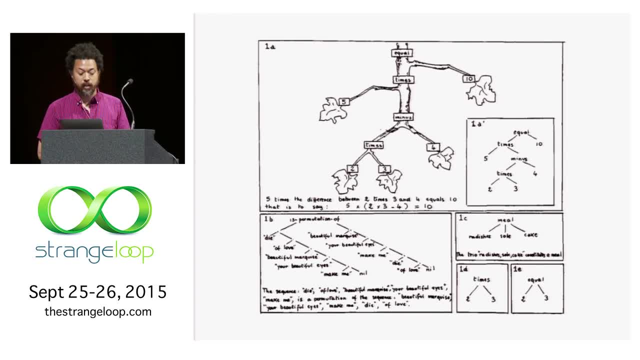 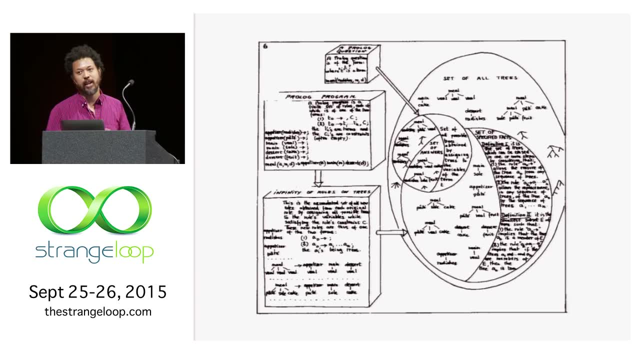 Really crazy stuff. I think even to this day we still haven't come to terms with the full psychedelic potential of declarative programming. So these are some drawings. These are drawings that Elaine Komarawa made, sort of describing how Prologue works and 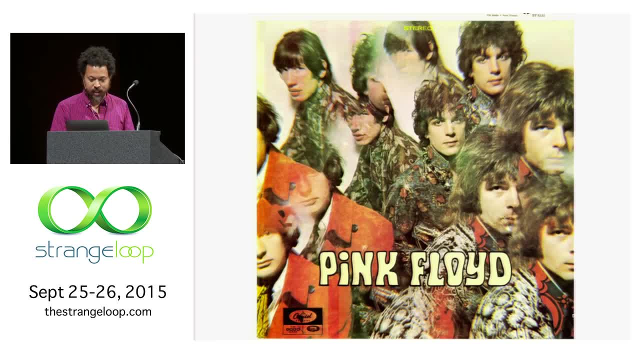 I like them because they just look like art and they're pretty crazy. So something to kick off is a band that I'm sure everybody's heard of: Pink Floyd. Everybody's heard of Pink Floyd. I'm not sure how many people have heard the early stuff that included Syd Barrett and 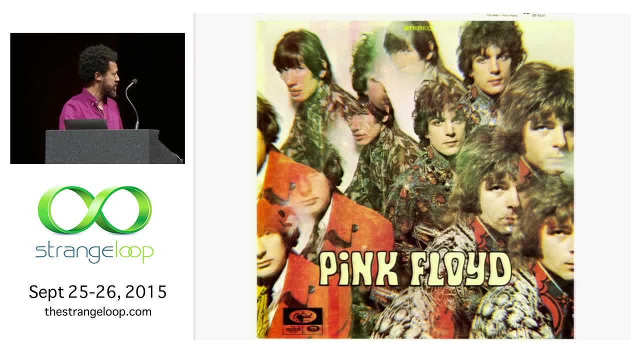 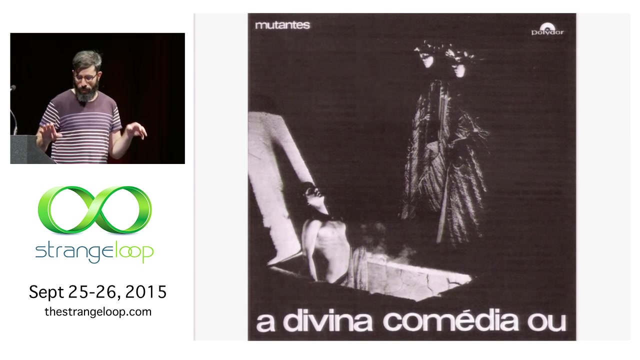 so we thought a good tune to kick off this section is Lucifer Sam off their first record. All right, that's it in the middle there. So one thing that we wanted to make sure that we got across in this talk is that there's something really obvious and limiting, in a way, about the history of programming languages. 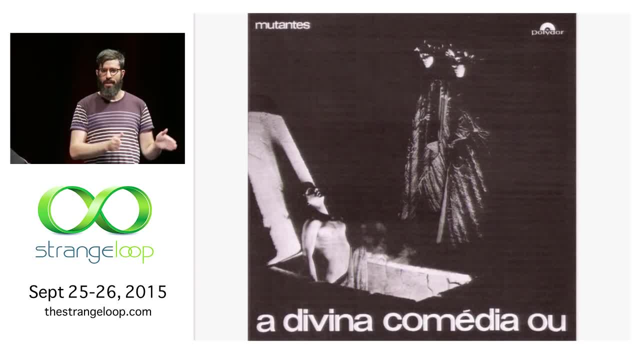 and programming language theory, which is that they all kind of came from people with very similar backgrounds, in very similar situations, trying to solve very similar problems. And a cool thing about music, as David noted earlier in the talk, is that it's universal. 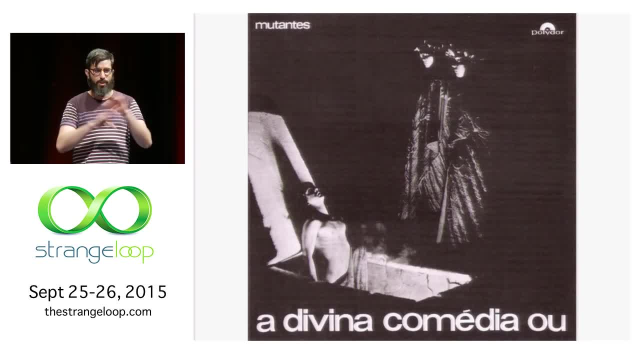 right And a cool thing about the 1960s is that It's universal. Yeah, This cultural change, the sea change that was happening, was not only happening in the United States, It was happening all over the world and there were amazing cultural, socio-political movements. 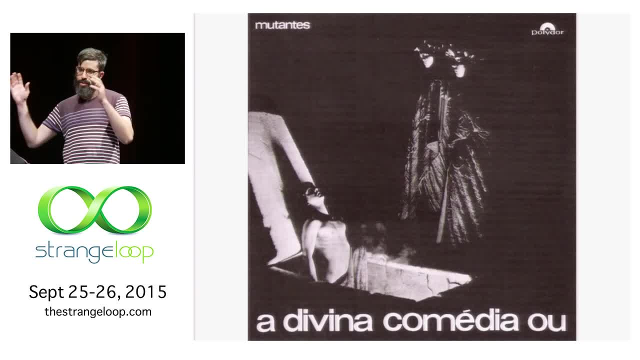 that were consuming countries in Europe and South America and Africa and everywhere, And one of my favorite instances of that was in Brazil. There was a new socio-political artistic movement called Trapacalha, and at the forefront of that was a band called Os Mutantes. 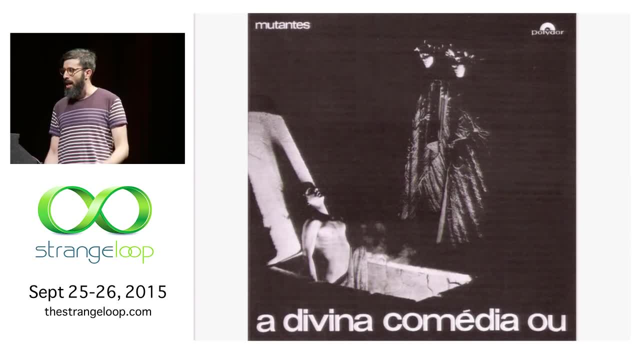 This is one of my favorite tracks from one of my favorite records of theirs, and what I want you to think about is that You know this uses the same substance. it's made up of the same stuff that Pink Floyd is right. 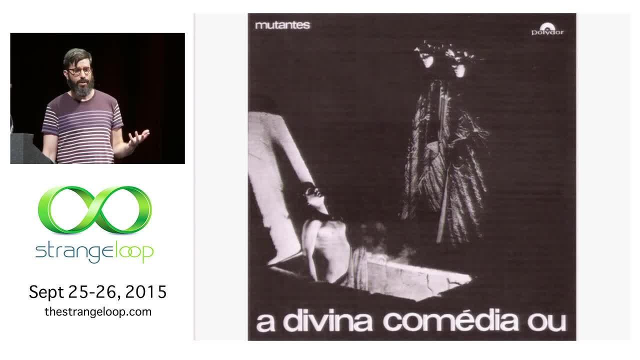 This is essentially the same instrumentation, although it's sung in a different language to express a very different purpose, toward a very different end, and we just think that that's beautiful, And so we wanted to share this with you to remind you that there's a lot to be gained. 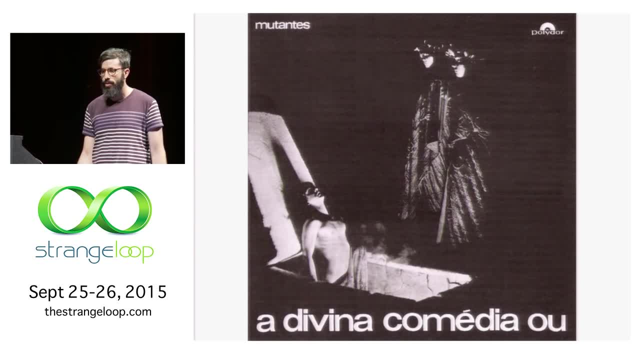 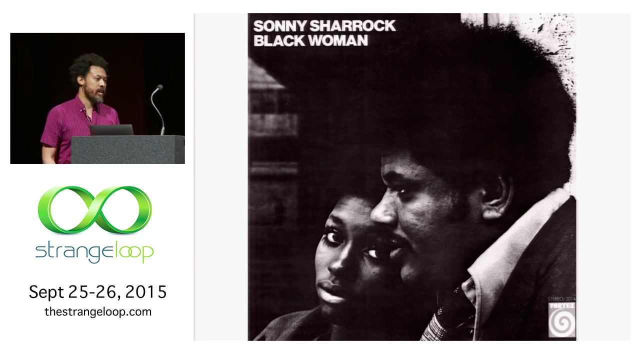 when you seek perspectives outside of the narrow scope of what you're typically exposed to. So here's Os Mutantes, The Mutants. We've listened to these samples so many times, Whee. This next one is, I think when, Mike, again when we got together to plan this talk. 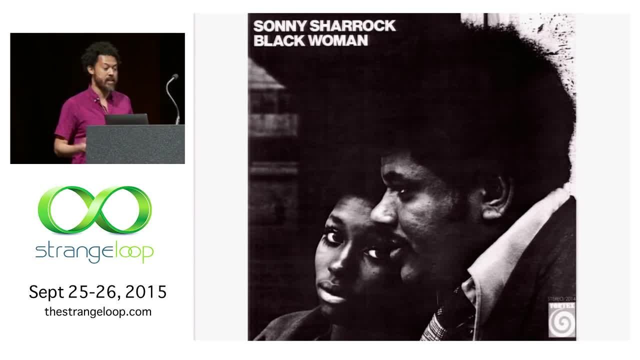 you know we have- we share- a lot of similar tastes. We also have different tastes, But one thing we agreed upon was this record: 1969, if you're a record collector- is one of the most amazing years ever in the history of recorded music. 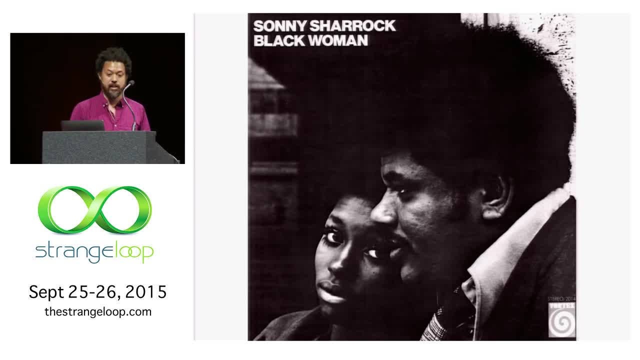 But this is a record I'm sure that you've probably never heard of. This is Sonny Sherrick. He is often categorized as a jazz musician, though I think the type of music he did was far more powerful than that. We're going to play you a track. 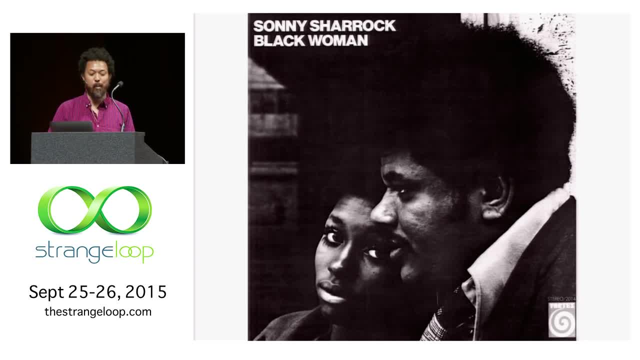 It's called A Portrait of Linda in three colors- all black. Do you have anything else to say about this track? I can't believe we're showing this to this audience And we're going to play them this right now. I'm so excited. 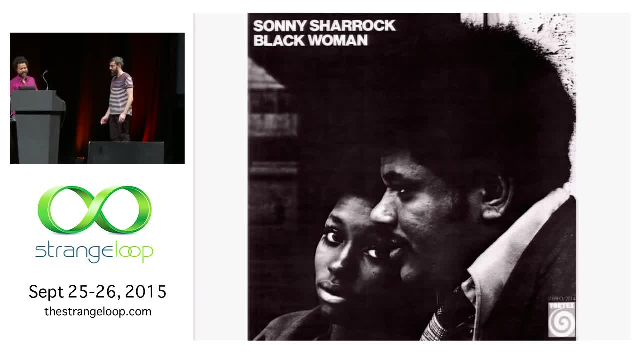 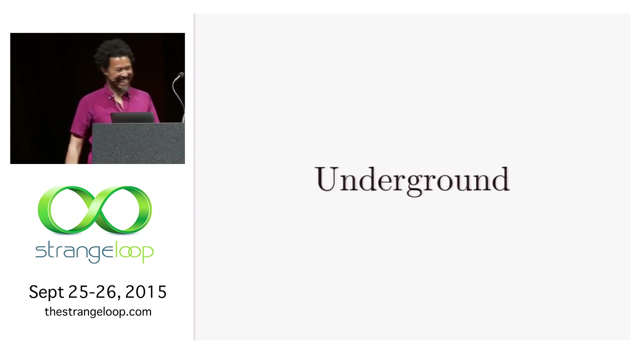 So not much else to say, Just enjoy. Oh yeah, guitar solo. So nothing happened in the 70s. We're not going to talk about it in the 70s Next, So we're skipping to the 80s. 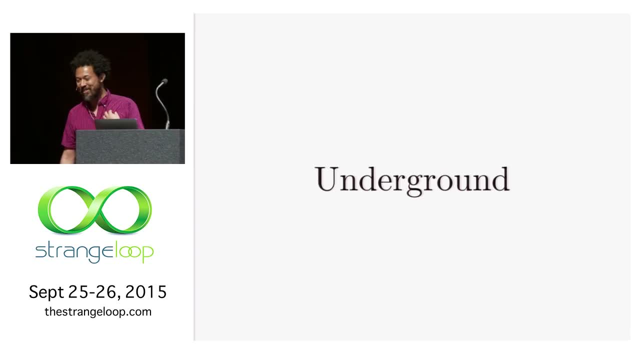 Because we can, It's our mixtape- Make your own. You like the 70s, It's cool, Make your own. So the 80s, I think, are sort of remembered for rampant commercialism. I think, Mike and I, we both love pop music. 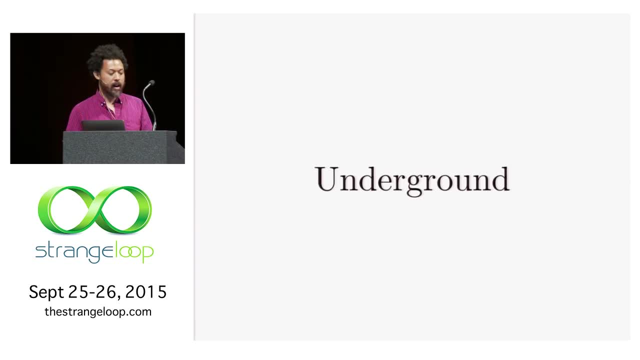 I mean, you know Michael Jackson, Madonna, Cyndi Lauper, that stuff is great. But what was cool, I think, about the 80s was that really it happened in the mid-70s really. 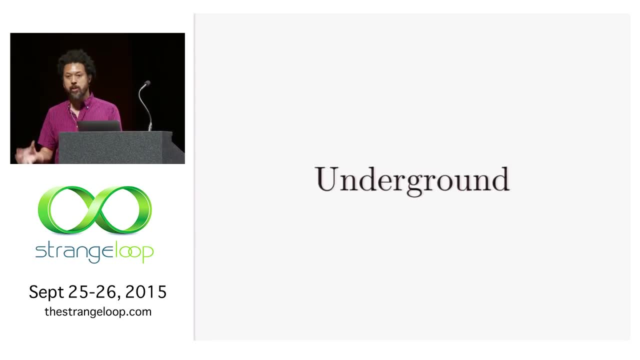 but the beginning of what you could call independent music and underground music. What was happening? in a similar way that computing was becoming very cheap, the materials required to record a record was also becoming cheap, and artists could take matters into their own hands. 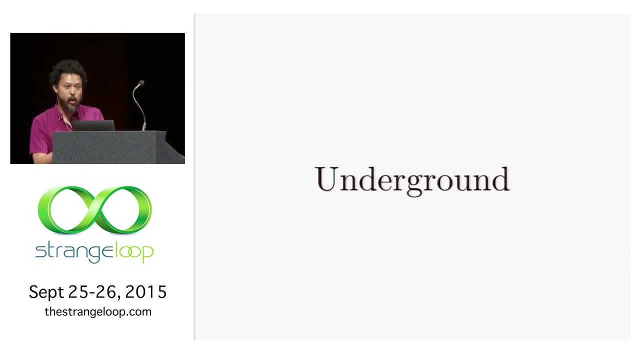 So we're going to focus first on some language, Some languages that we think were underground- And what's interesting about what's once underground often becomes mainstream or has a far bigger influence than anybody could imagine, And I think these programming languages really fit this idea. 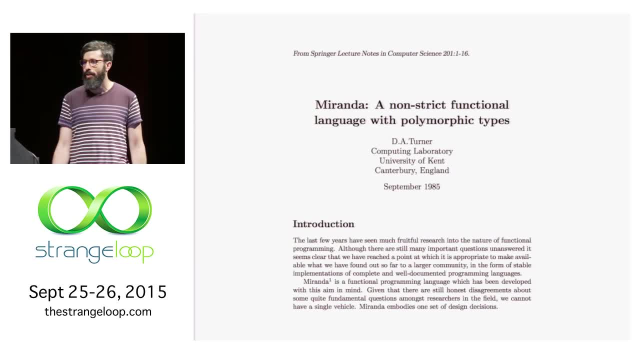 So the first of those that we're going to talk about is a language called Miranda, developed by David Turner. This is a paper from September 1985. And it's called Miranda: a non-strict, functional language of polymorphic types. 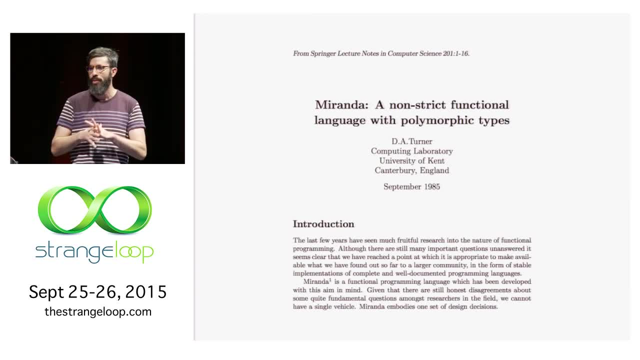 And some of us write code in programming languages that still don't have access to these features, Right. So, as David said, this is an idea that ended up having a very long shadow. What's cool about Miranda is that it's lazy. it's a pure functional programming language. 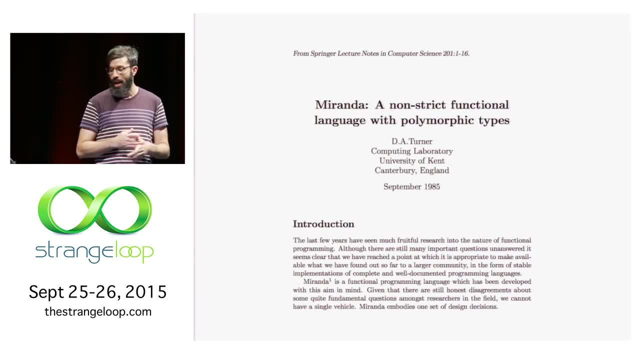 and it was the predecessor, the spiritual, direct predecessor, to Haskell, a programming language that we both love, And it is just incredible to see at this time the sort of nascent form of these ideas that a programmer interacting with a computer could get a lot. 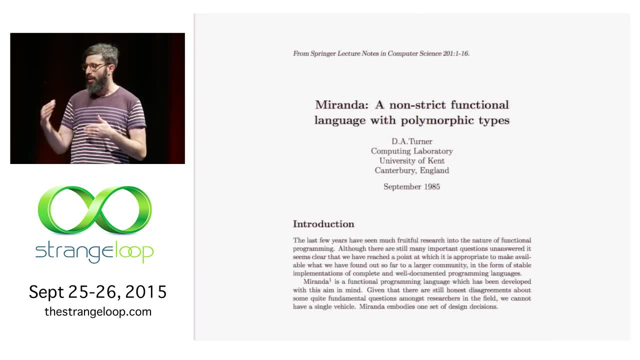 of assistance from the computer in writing programs and could lean on a type system and think about things like referential transparency and its impact on your ability to express programs. So we really wanted to choose this because it's a language that not a lot of people know about. 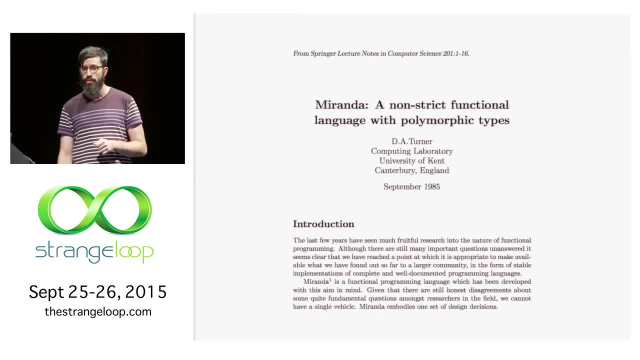 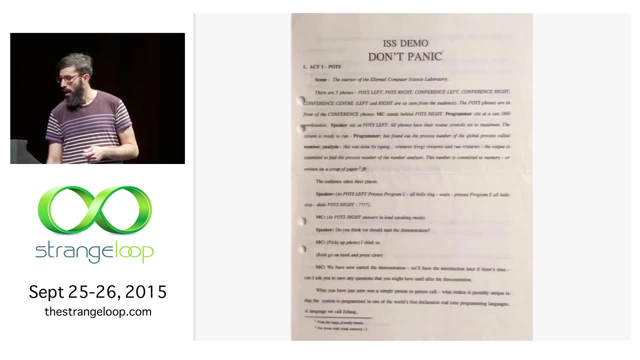 and one that you should check out if you want to know where some of the roots of some of these languages that you may hear about a lot come from. Miranda is a big inspiration to those, And next we have here the Joe Armstrong was kind enough to tweet this the other day. 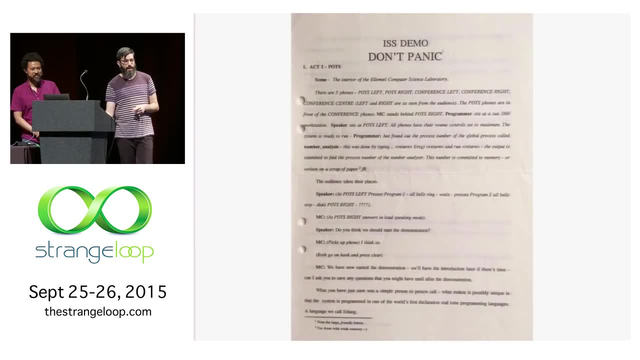 This is the first page of the script for Erlang, the movie. And so, and yeah, what up, Joe? So Erlang is another amazing, really interesting programming language that still struggles with its undergroundness in a way. right, 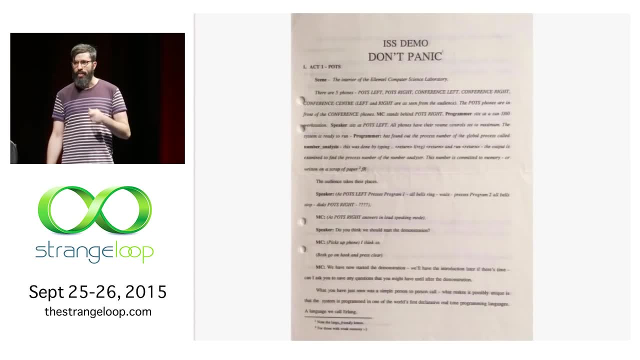 But the reason why I wanted to bring it up here is because I think what's so amazing about it is that it's designed for a very specific purpose. right, It's a language that was designed for a particular domain, and it did it really well. 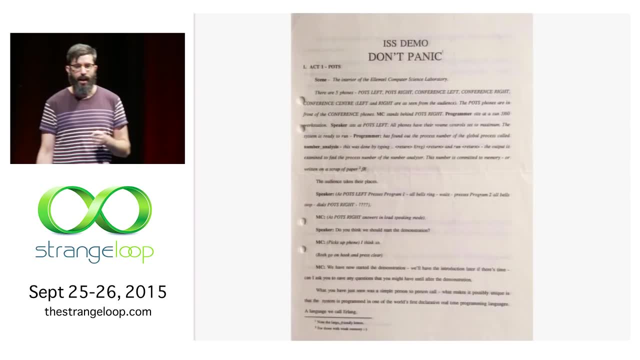 or actually it does it really well, right, still doing it. Ericsson, where this language was invented, still employs this language to run its telecommunication systems, with 99.N9's uptime, hot code, reloading functions, modules and a lot of things that, again, you don't see in other programming languages, right? 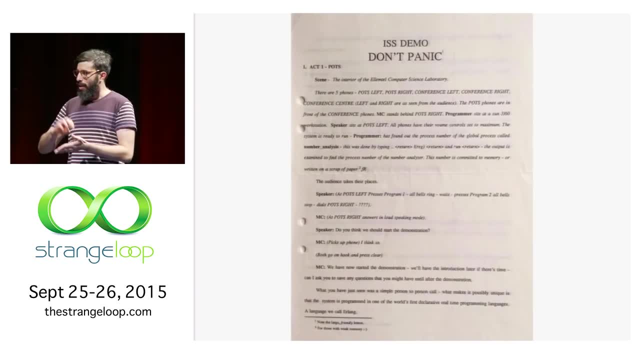 And it's just this really interesting thing where, born out of the desire to solve a very, very specific problem, a very specific and a very successful solution was created, And though there are still some sort of specific purpose programming languages today like this- this, to me, is one that really stands out, and Erlang is a really cool programming language. 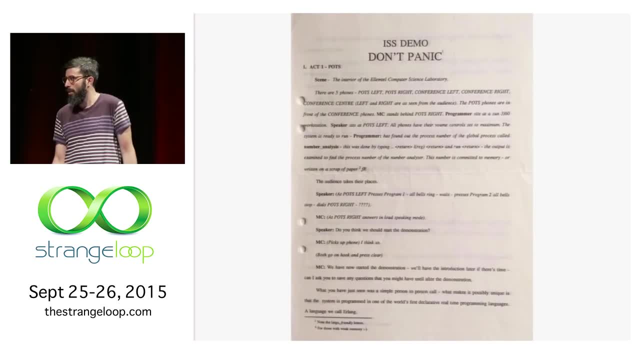 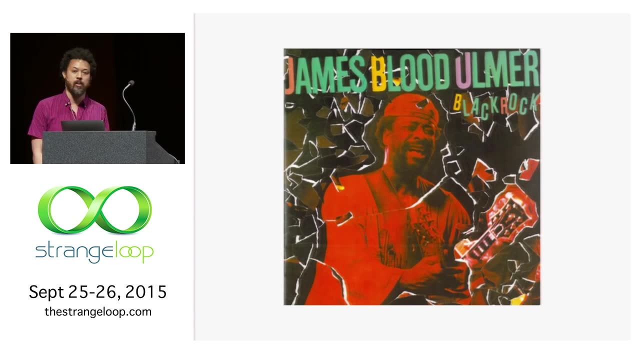 that we're also fans of. So for this section we picked some things that you're unlikely to have heard anything, except for maybe the last one. The first thing is James Blood Ulmer. He was. he worked with Ornette Coleman. One of the coolest things about his guitar style is he only plays with his thumb. 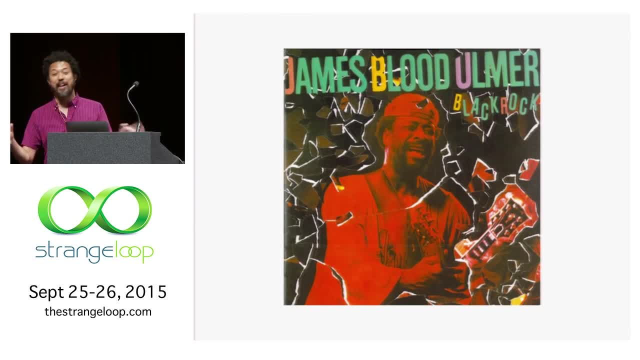 This is his band that he put together This record. this recording has like. you can find this in a dollar bin and I totally recommend picking it up. It's awesome. Do they have dollar bins anywhere? Is that a thing? Does iTunes have a dollar bin? 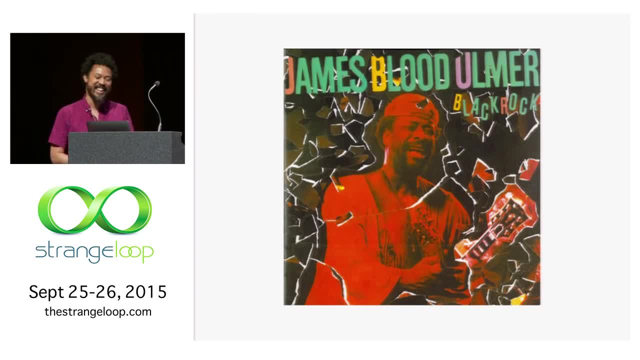 Right, right, You could probably get this for three bucks on iTunes. It's just a weird record. It's like funk, it's soul, the R&B punk. I mean it's all mixed into this crazy thing. Very short clip. 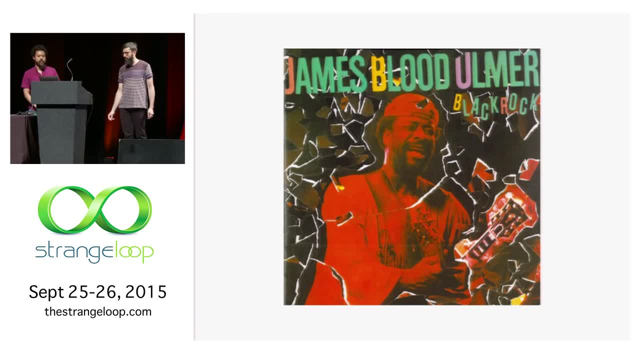 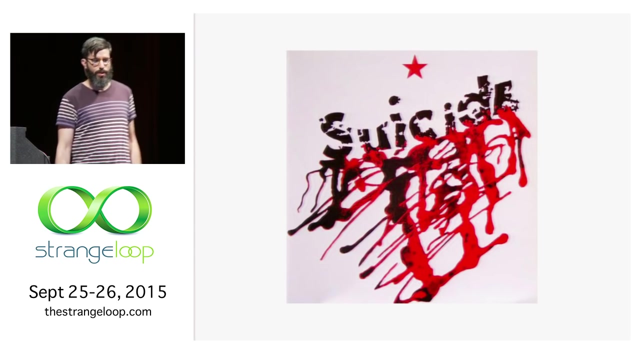 And the next thing Mike's going to talk about- Yeah, so toward the end of bands that were influential but that a lot of people may have never heard of, is a band called Suicide. So this is a band that was around in the early 80s in New York. 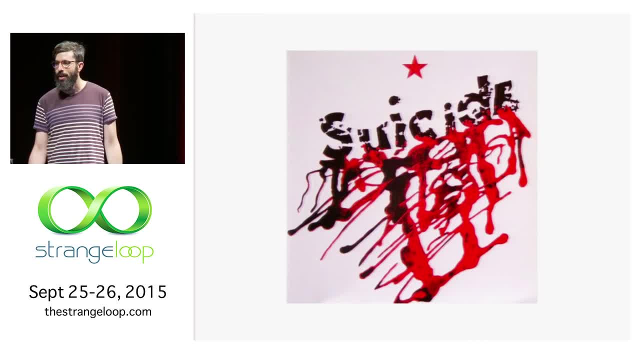 One of those records that you definitely didn't want your parents to find in your bedroom when you were a teenager, because then they're going to ask you a lot of questions about the name of the band and the violin cover. But this is a really cool record because it's two people, Alan Vega and Martin Rev- and 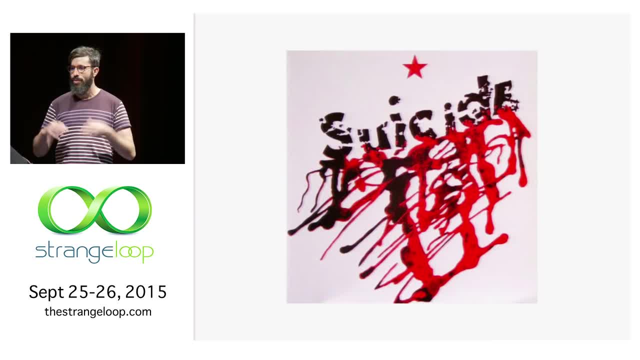 they're trying to make a new sound. They're in a time and place where there's a lot of very interesting music happening. The end of disco Around the time of post-punk movement, Post-punk had sort of been in full swing. new wave hadn't really happened yet. synthesizers: 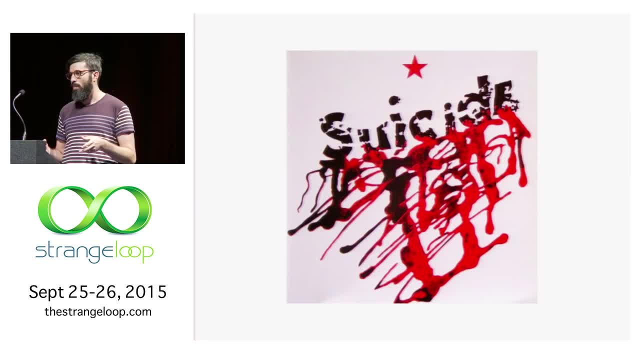 weren't uncool yet, And they did this thing where they wanted to play music that represented their time and place and were known for these kind of very aggressive live performances. This is a track off their album- their first album- and it's called Ghost Rider. 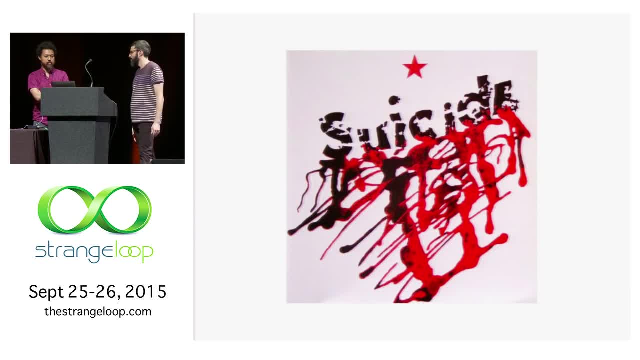 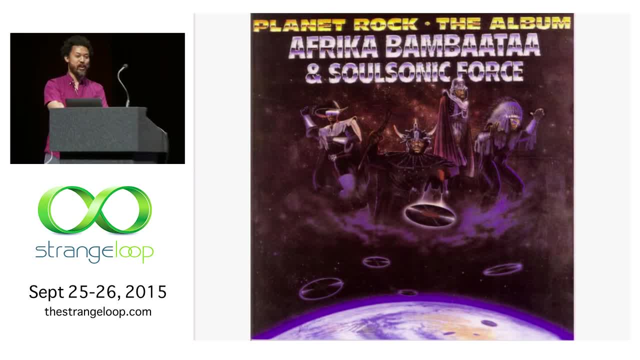 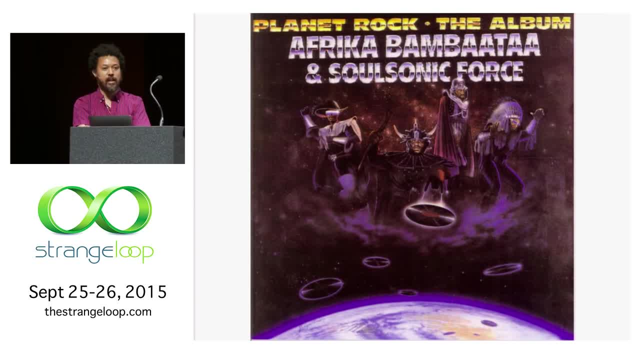 about. It was just something that happened at parties in basements. It wasn't yet a worldwide phenomenon, So we thought we couldn't do music justice if we didn't pick this. What I like about hip-hop, though, specifically, is that you'd reached a point in recorded. 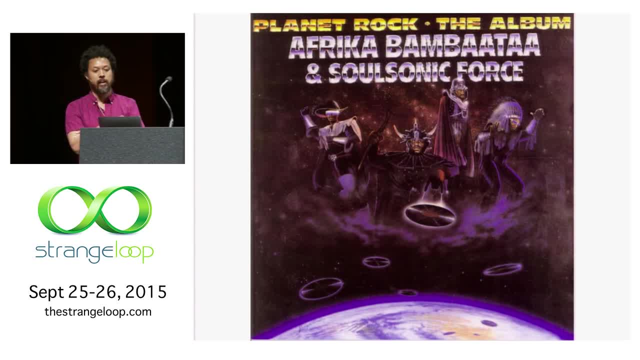 music where there was so much prior stuff to sample that you could make music purely out of samples. This piece actually has a really great reference in it, which is they take the keyboard line from a Kraftwerk song and Kraftwerk is kind of an amazing early electronic sort of kraut. 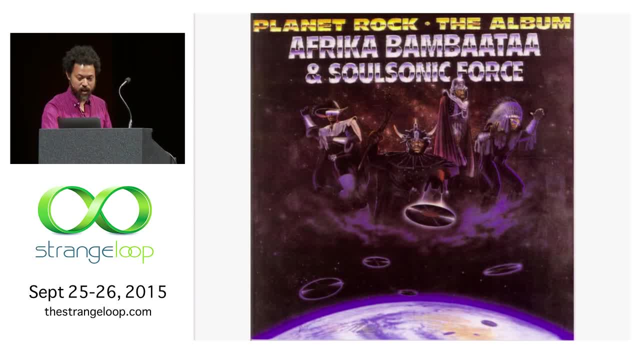 rock band, which is also really good, but this track is pretty awesome. So same with the 70s. nothing happened in the 90s. Actually, something happened in the 80s. I don't know, I don't know. 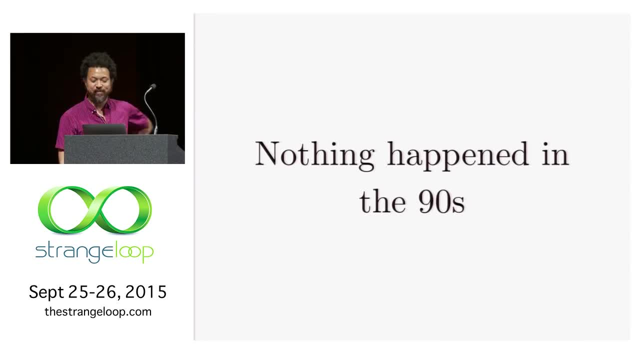 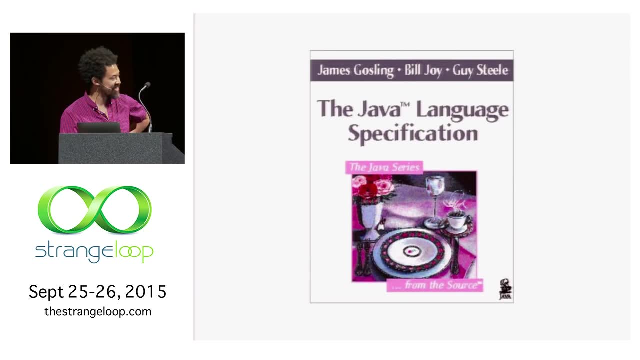 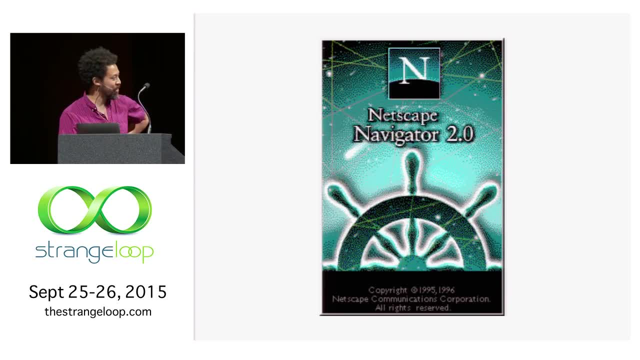 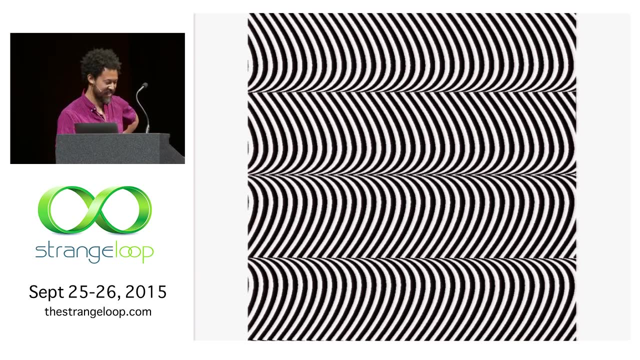 Java happened in the 90s, JavaScript happened in the 90s, And we think there's a really good tune for this fact that these things happened. I didn't see anyone dancing, So that was a piece by a Japanese noise musician named Merzbau. 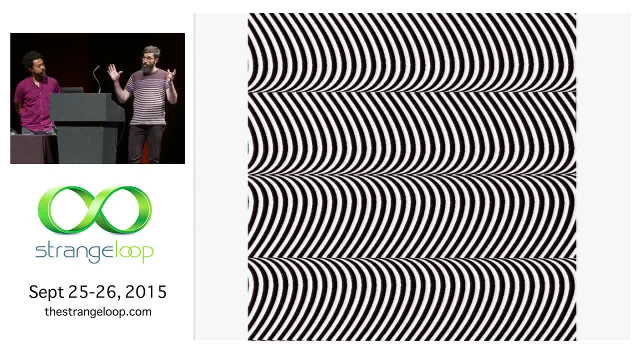 This music was created in his bedroom, Right, And the cool thing about this is that the thing about hip hop was that you know so much music had happened up until that point, so they decided to kind of utilize that in an interesting way by sampling it and referencing it. 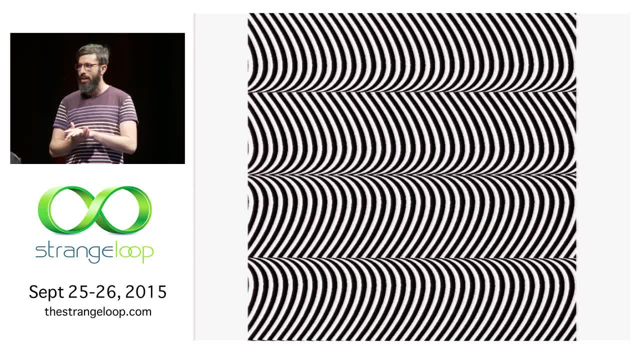 On the other side of the coin you had people that you know understood the fact that so much music had happened up until that point that they just wanted to destroy the actual notion of music. Question: what is music and what is organized sound and all of these kinds of things? 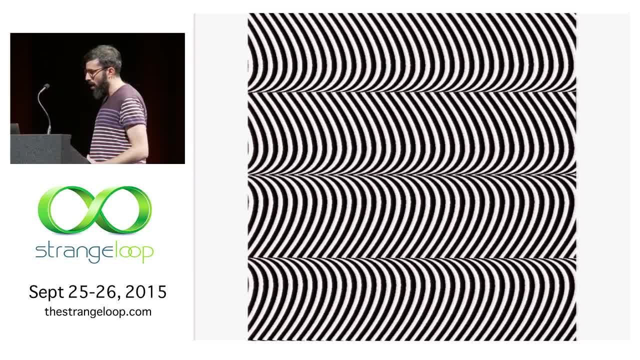 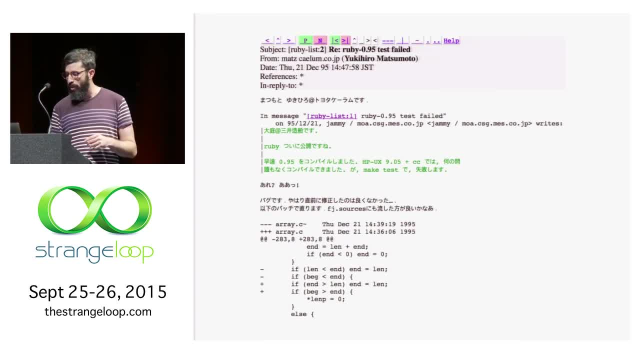 So, similarly, around the same time, you have people who are really interested in music, Right, And you have people making programming languages in a different context from the way that they were normally made. So here's the mailing list post from December 1995 by Yukihiro Matsumoto, and he's talking. 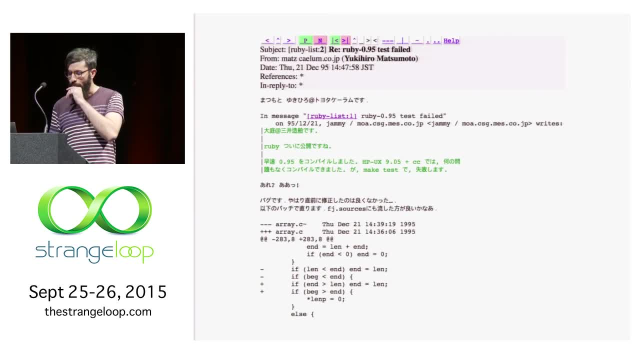 about a language that he's playing with called Ruby and it's, you know, meant to replace sed and awk and purl, and you can do some really interesting things with it. And you know this is a mailing list post on the Internet. 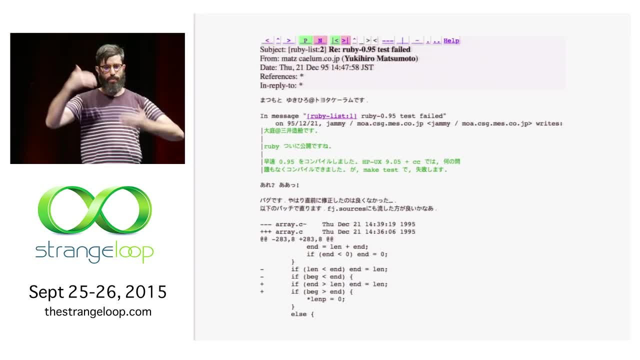 Right, And all of the other languages that we showed you were like academic papers, Right. So we thought that that was really cool, And there are a lot of other examples of this. We noticed this when David and I were kind of. we collected way more material for this. 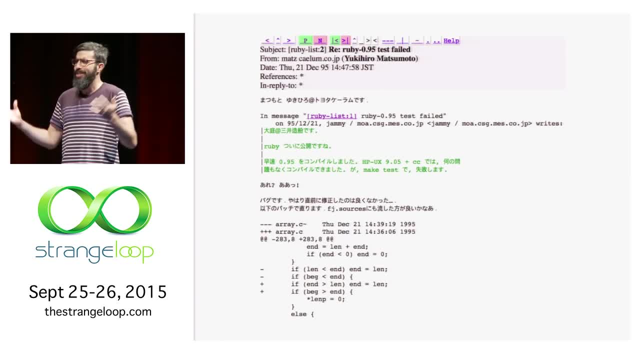 talk than is actually in the talk, and by the time we got to the 90s we're like. all of these languages were announced on news groups, including Python, Perl, Ruby, Clojure. There was a post to a Java mailing list or something like that. 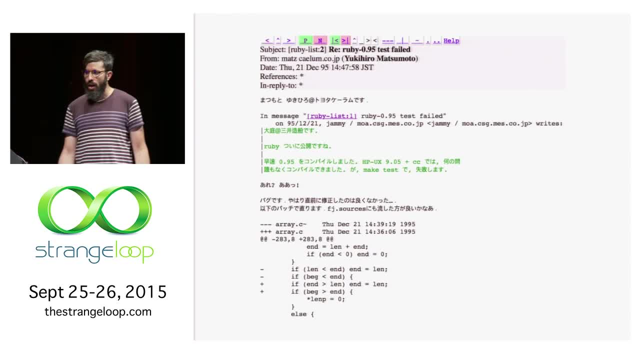 So we thought that that was a really interesting thing to point out, Sort of on the end, sort of toward the end of you know, this is the natural consequence of an underground movement happening is that, you know, proliferation of material and things. 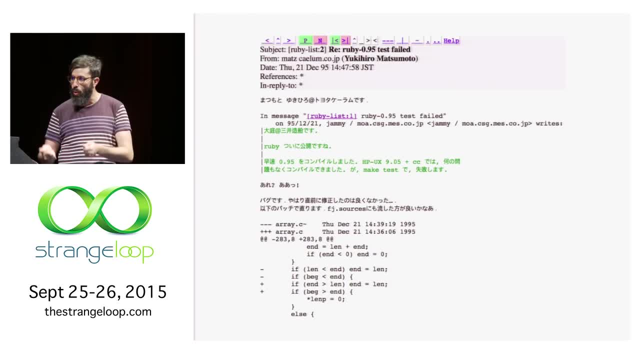 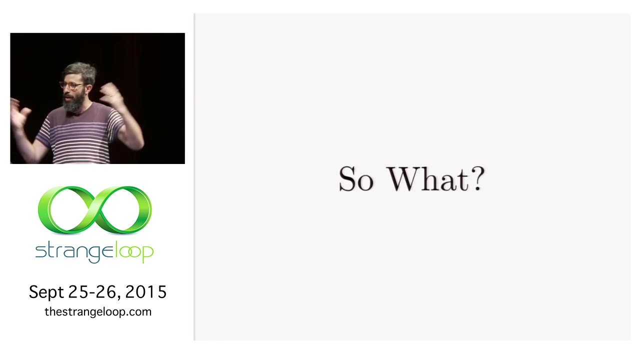 being easier to use, and people having access to more material means more better things are produced, because more diverse perspectives are included, And so that was something that we thought that was really important to point out. So what? That's the end of our mixtape. 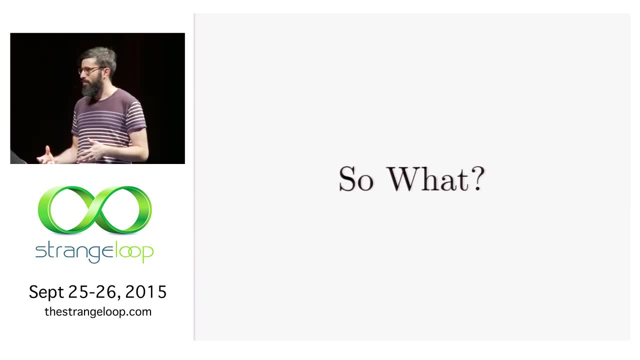 But we wanted to make sure that we didn't end the talk without trying to tie it all together a little bit. So I have my own ideas about so what. But what about you, David? So what? So for me, I was, you know, when we were at the end of coming up with what this talk was. 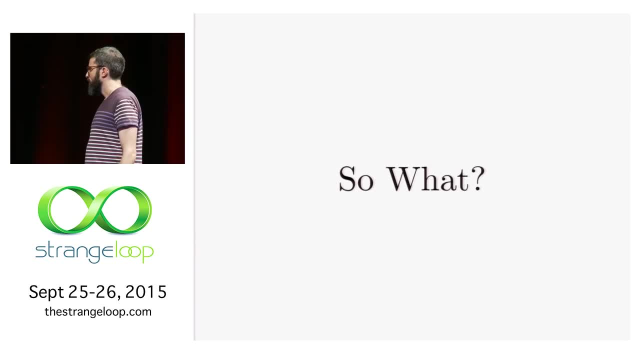 going to be about when we sort of saw the slides and had all the music. a theme that came up every time we talked about the material was that as sort of fans of music, you know, we both had kind of agreed that if people just saw the slides and had all the material, 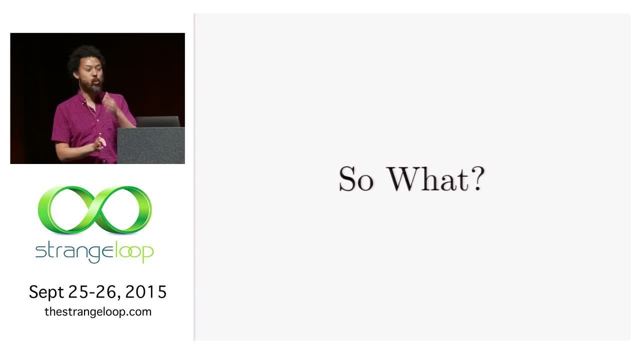 if all composers stopped making music, you could never go through all the awesome stuff that's been done in the 20th century. It's not possible. At the same time, we feel the exact opposite way. with computer programming and programming languages It's like no, we can't stop now. 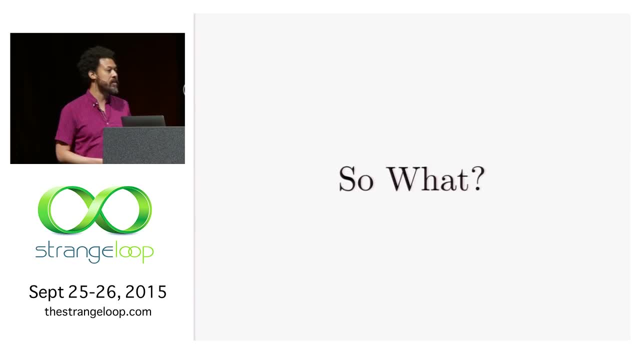 It's not time to stop. It's just so much more work to do, And a lot of this is, I think, in some sense while recorded music changed the way we feel about music. music is really old, right, Thousands upon thousands of years old. 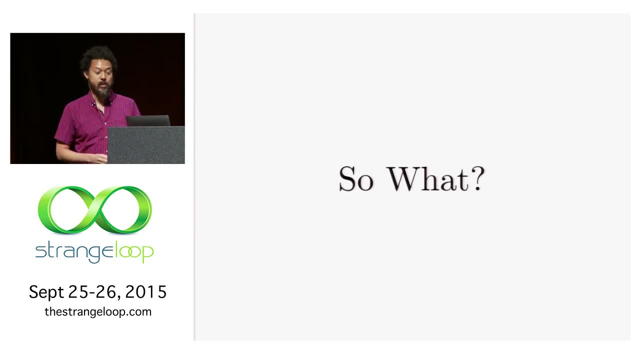 thousands of years old. We don't even know how old it is. So that's my take And yeah, and I think another, I think to add a little bit to what David said. so what, like, if you think about the infinite amount of amazing music that has been created by 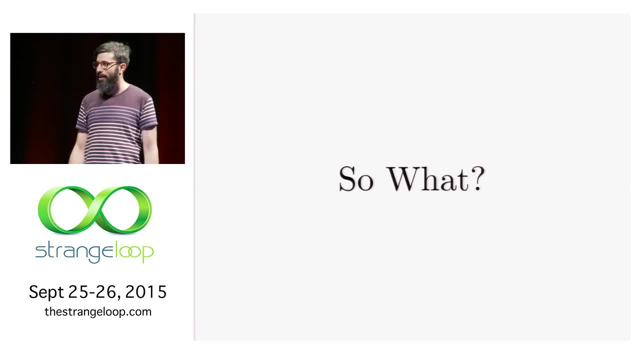 humans all over the world throughout history and the unbelievably rich tapestry that that creates. that's what we should be striving for when we're creating programming languages. We should have programming languages that represent every diverse perspective, that come from every place, that are born of any kind of environment.